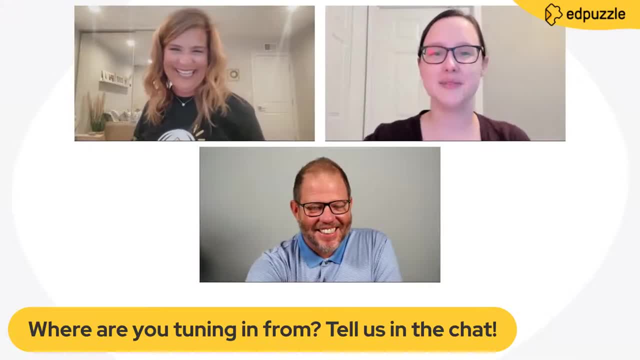 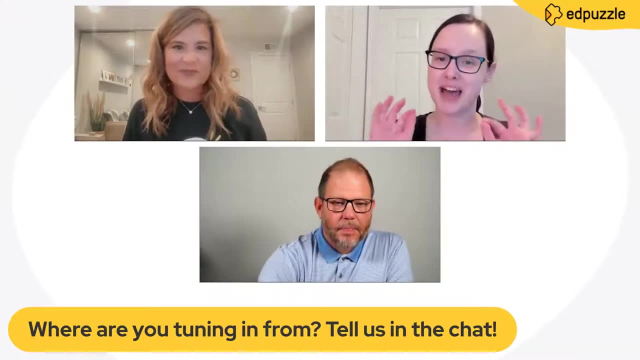 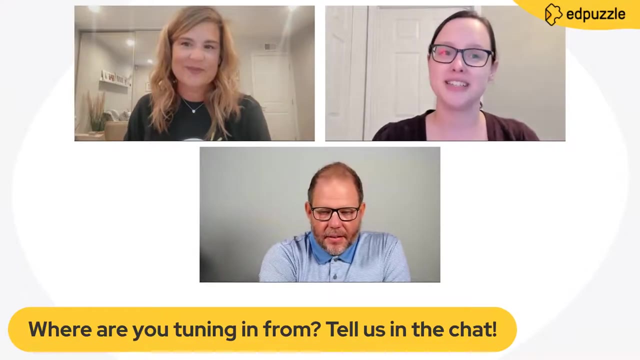 going to talk about you. Yeah, So, Graham, he's been an educationist, classroom teacher, a math instructional lead and currently as a math specialist. So we have a math expert with us this evening. He's continually advocating for best practice in elementary mathematics by seeking new 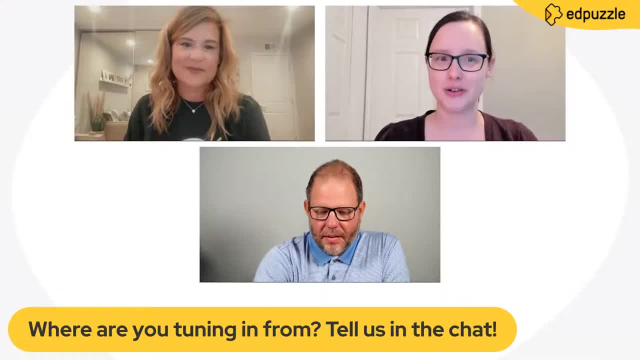 and innovative methods to improve math, And he's also been a professor at the University of New York and at the University of Chicago, So we've been very excited for him. So, Graham, please share some of your innovative ways to support students and teachers in their development of conceptual 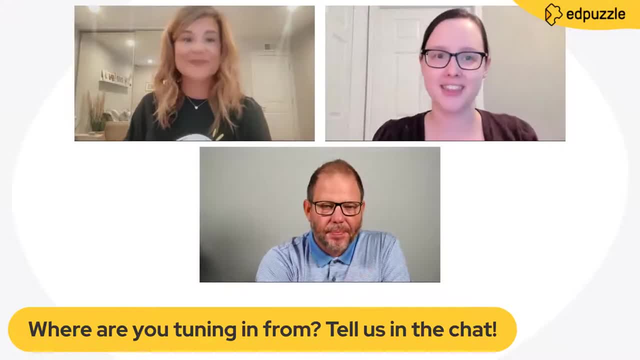 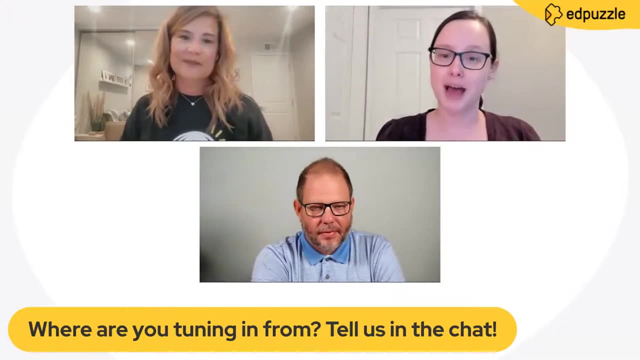 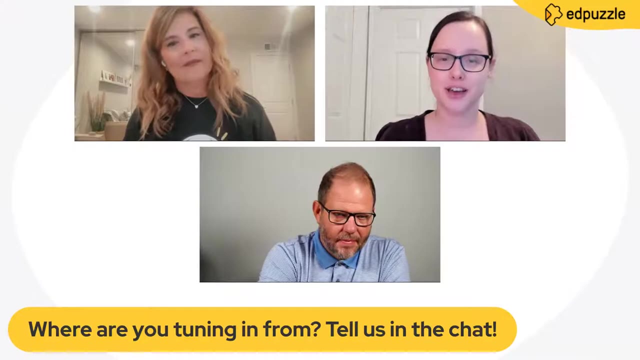 understanding, which, in math, is so critical to being successful and competent in math. He's the author of Building Fact Fluency, a toolkit for addition and subtraction, And you can find him on the web at gfletchycom, on Twitter at G Fletchy, or on Facebook at facebookcom. slash- G Fletchy. 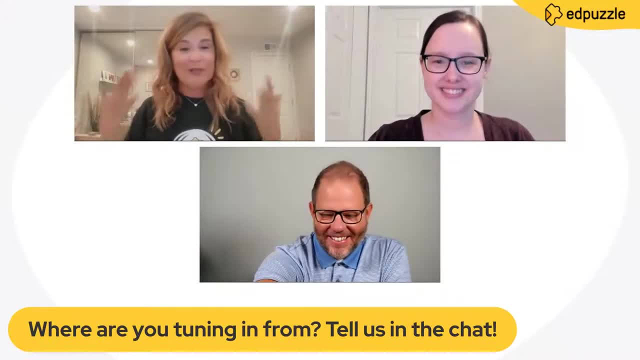 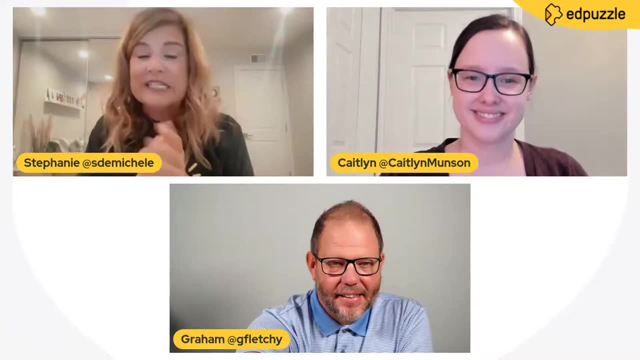 Okay, math phobic. I am a confirmed math phobic. I'm looking forward to this. I brought my paper, I brought pens. I'm ready to do some stuff. So all of you who are out there, please don't hesitate. 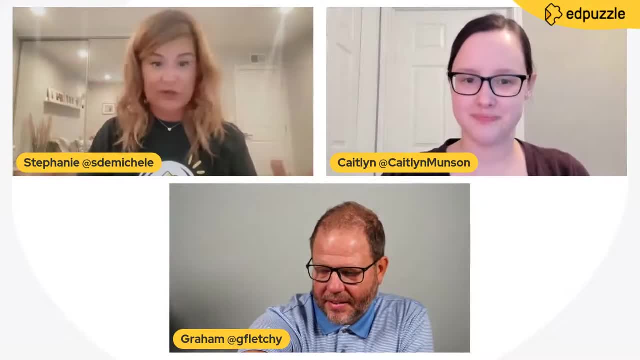 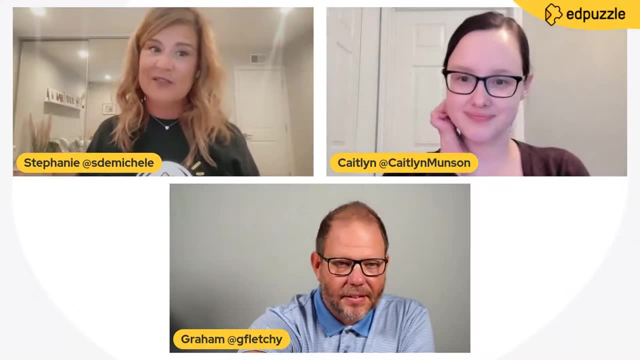 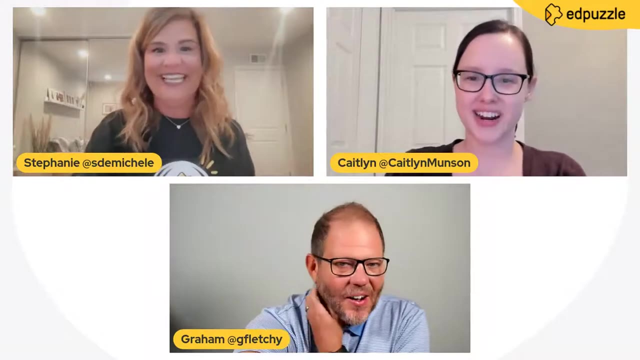 to ask questions while Graham is going. you know sharing his workshop, share your own experiences, share your aha moments, And if you are evangelizing this event on social media, please don't forget to use the hashtag EdPuzzleLive. All right, So we're going to kick this. 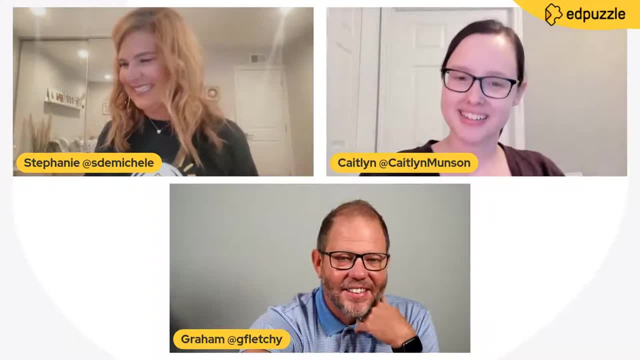 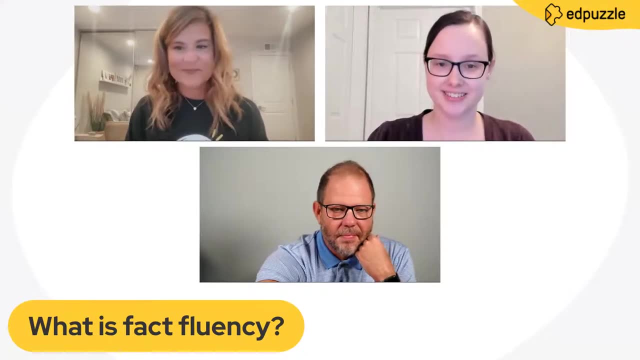 off. So welcome Graham, And if you wouldn't mind explaining it to our audience before we get started, what exactly is fact fluency? Because that's what we're here to talk about tonight. Yeah, So awesome. Well, thank you, Steph, Thank you Caitlin, Thank you to Manny, holding the 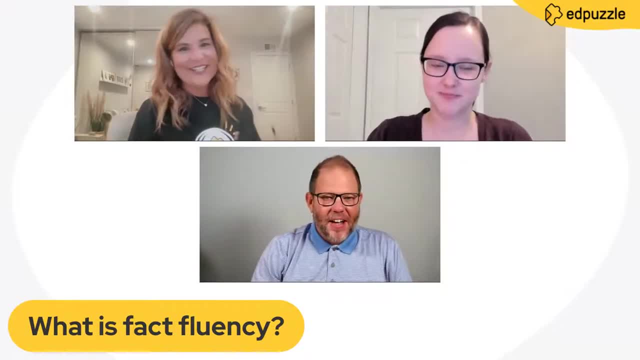 fort behind the curtain, the wizard behind the curtain. there, It means a lot to just play in this virtual space with you all. So, fact fluency: I start thinking about what fact fluency is, and it really means a lot of different things. 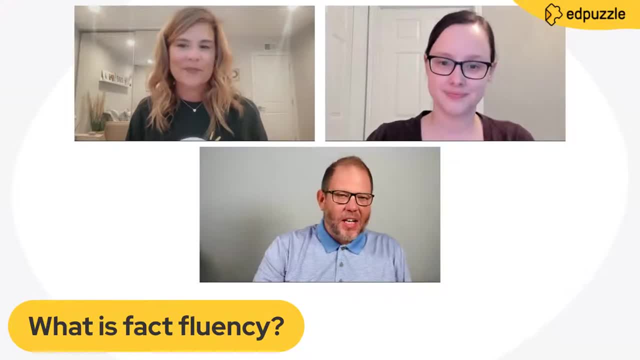 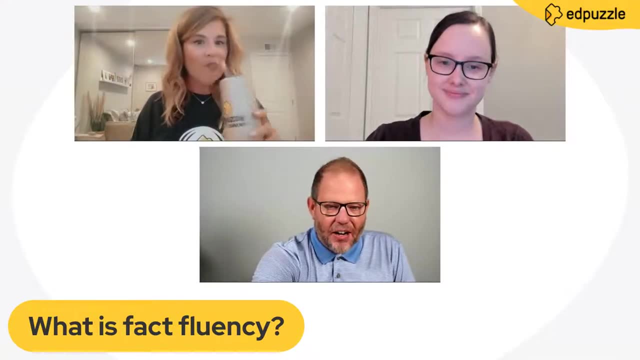 To so many of us, So let's just not waste any time. Let's jump in. We've only got a short period of time here, As I was sharing with the team before we got started. it would be like drinking from a fire hose today, So let's not waste any time. I'm going to go ahead and share my screen. 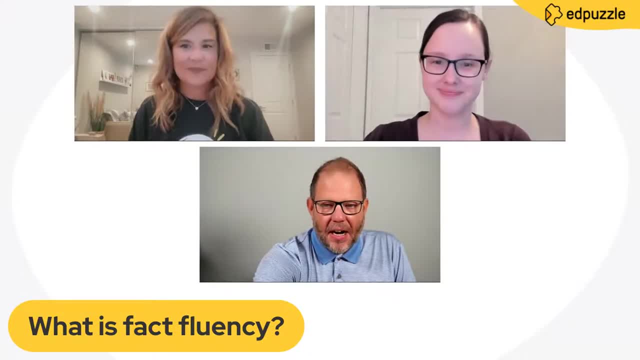 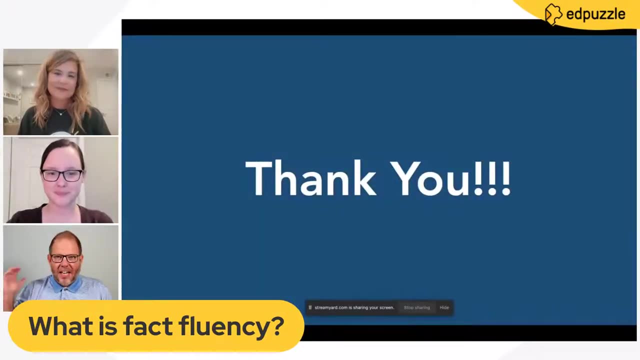 And, as I share my screen, we're going to talk about what fact fluency is and also what it can kind of look like and how we can approach it differently in our classroom. But before we get started, thank you to you. whatever you needed to do to get into this space, whatever platform you're, 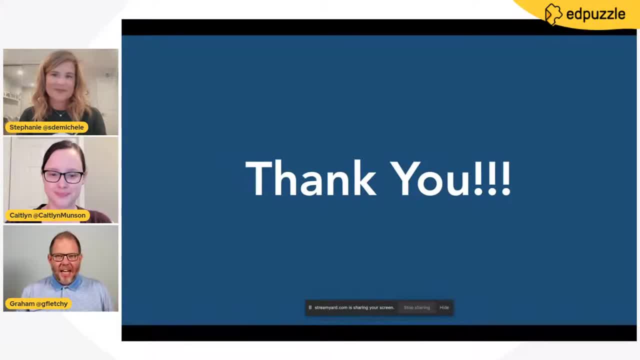 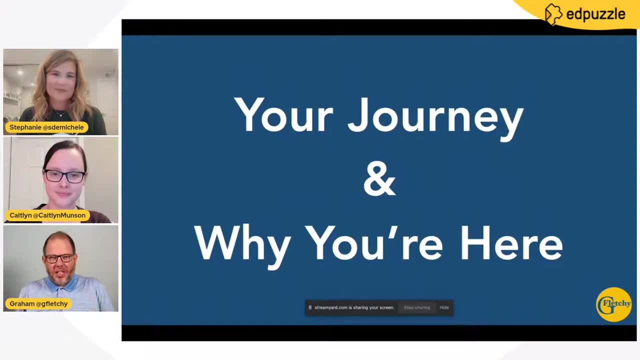 watching this on. Thank you for just taking the time out of your busy day, But let's be honest: whenever, if you're an educator of one year, an educator of 25 years, whenever you see or hear a session regarding fact fluency, you're like I've got to sign up for this right. I know I do. 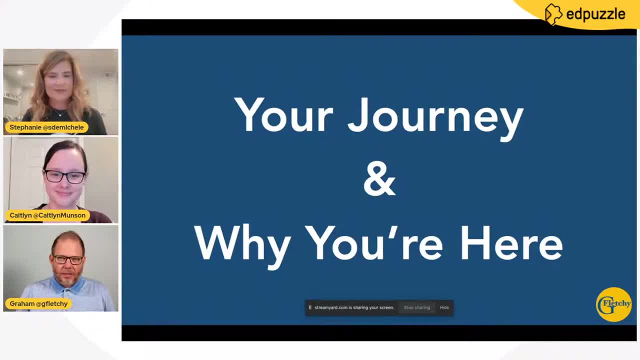 when I go to conferences, especially over the last couple of years, been lots of things on fact fluency in this virtual space. So I think about this, though It doesn't matter if you're a new teacher or a veteran teacher- We've kind of thrown the kitchen away. We've thrown the kitchen away. 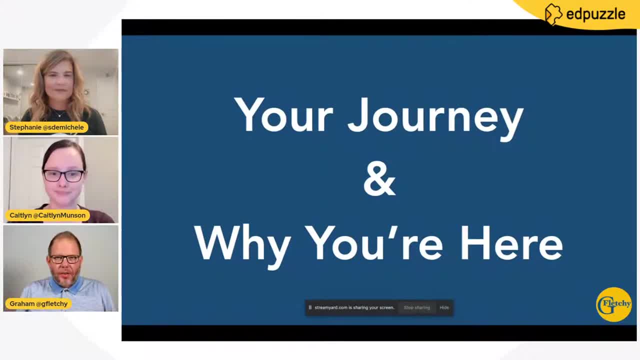 We're students, We want our kids to know their facts. All of us have kind of been in this place to where we've all probably said, myself included, like my kids just don't know their facts, where we have kids who know their facts on Friday and we're super jazzed and we go home and we have 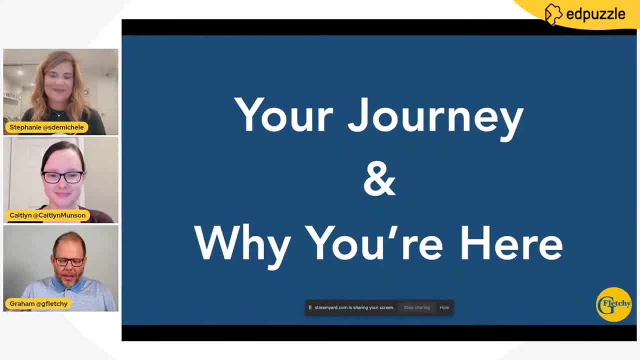 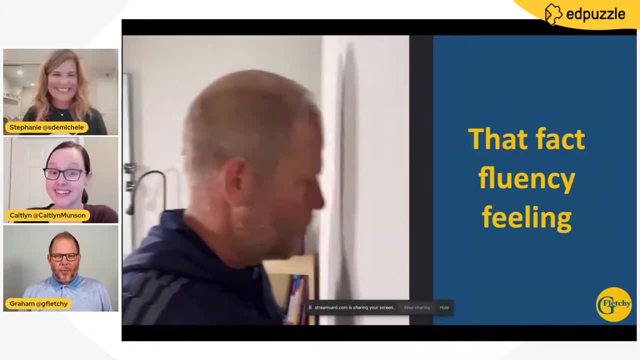 the best weekend ever and we come back and we're ready to build on that fact. fluency and kids have completely forgot their facts right, So it's like we go right back to square one. We're lost, We're frustrated, Something. 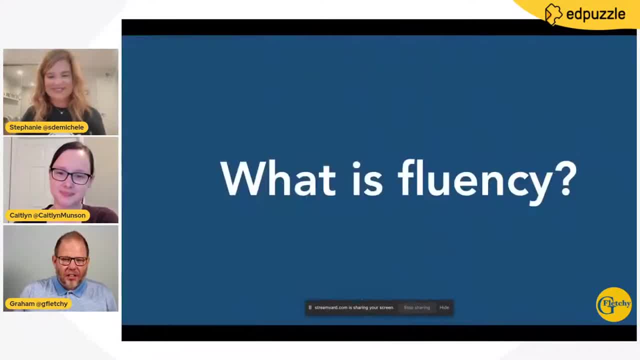 Right isn't sticking. So what I'd love to do is just in the chat window say: if a first-year teacher, a parent, a student, what's the first word that comes to mind when you hear this word- fluency. I'll sit tight here for about 10 seconds. What's the first word that comes to mind when you 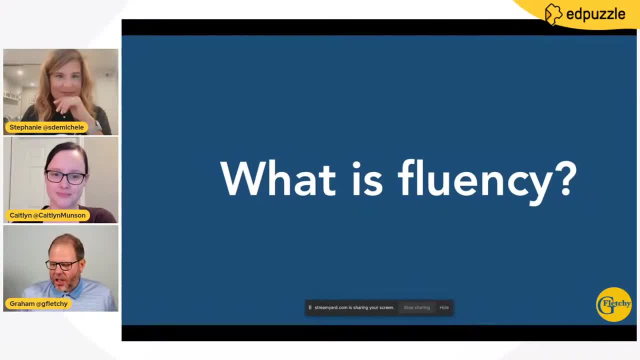 hear this word fluency or fact fluency. Jot something in the chat window for us, please, and thank you When they're doing that. I mean, I think of it in terms of language. Okay, You're fluent in another language. 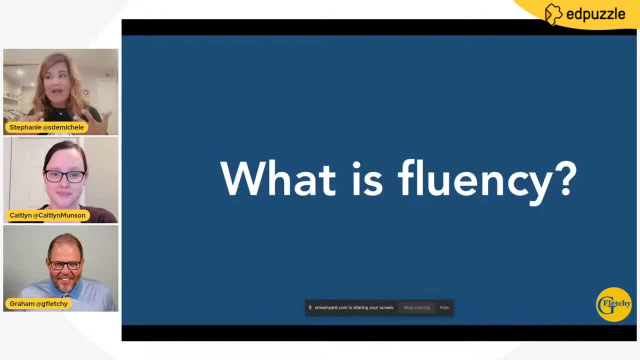 Yeah, Yeah, Which means I'm not thinking about what I'm going to say, It just automatically comes to me. Yeah, Like yes, we've got Again. it's just automatic. Yeah, Yeah, Automatic is what I was thinking. and then Kelly put it: Yeah. 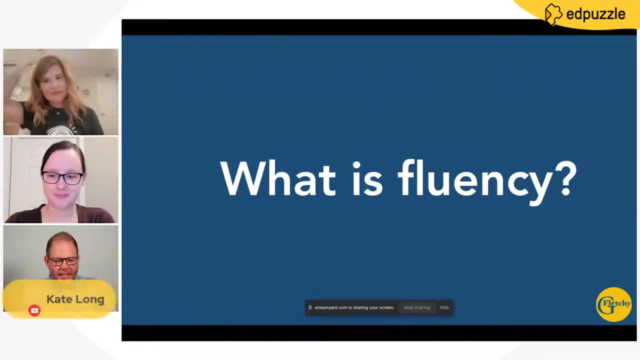 So I start thinking right Like as a third-grade teacher. I would need kids that could read 120 words in a minute by the end of the school year, and I would have kids who could read 150 words in a minute but they couldn't tell me a lick of what they just read, And in the same breath. 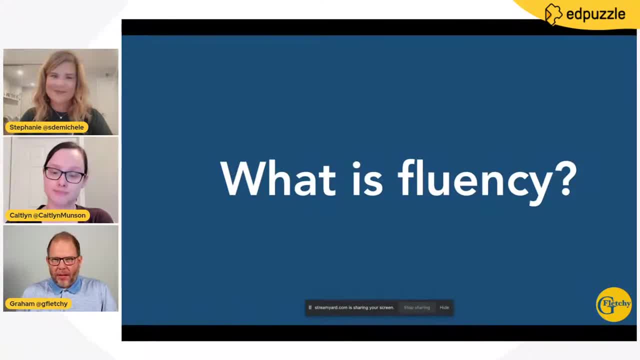 I'd have another student who could read maybe 70 or 80 words in a minute, And sure they might not have been as fluent, but they could make inferences and conjectures far beyond what the text was ever telling them. So before we get started, I want to tell you what I think fluency is. I just want to. 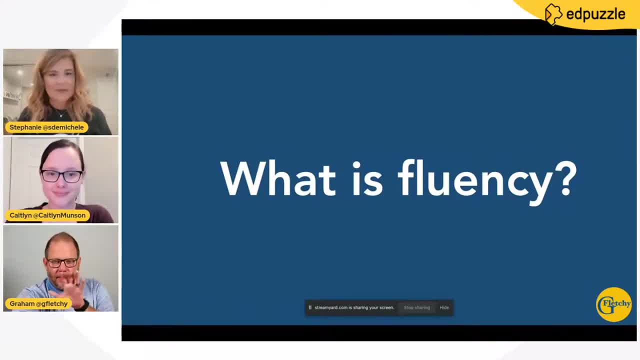 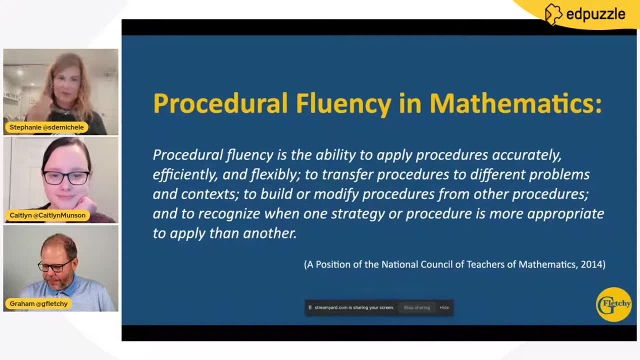 go on one piece of research, but there's tons of research that is completely aligned to this piece right here. I want to give you a quick moment to just kind of read this piece here. So if you've been playing around in the math space for longer than, say, a year, 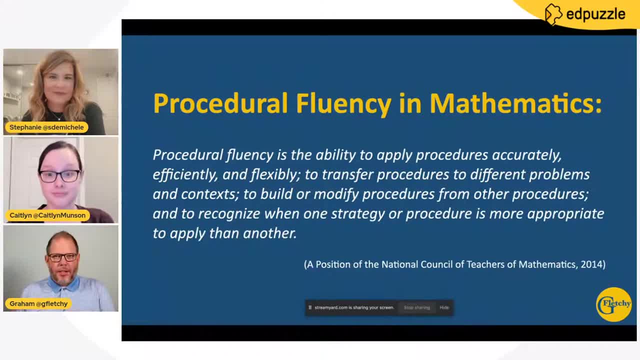 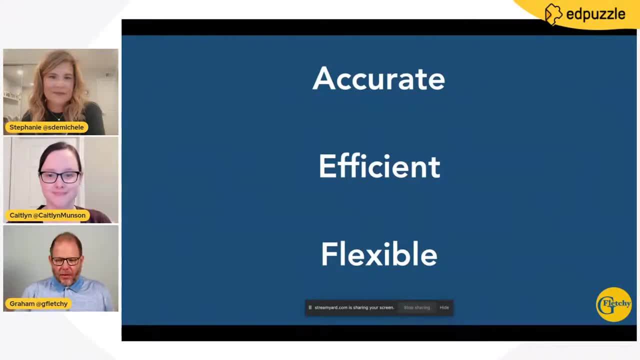 there's a lot of terms here that get brought up when we talk about fluency, especially in mathematics, And I know for me as a math coach and a math lead- these three terms get brought up a lot Like: if kids are going to be fluent, they have to be accurate, Like kids need to be. 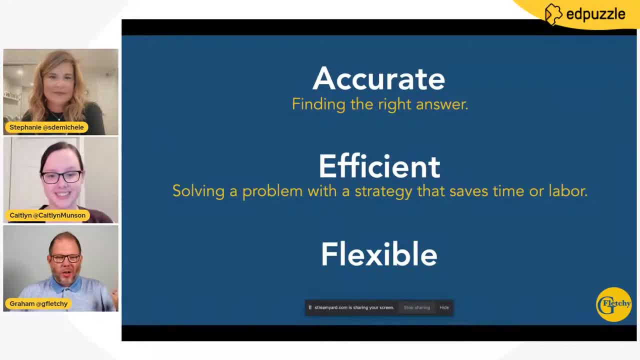 able to find the right answer. So if you're going to be fluent, you have to be able to find the. They need to be efficient. They need to be able to solve a problem with a strategy that saves time or labor. Like counting on can really stink when you are adding 53 plus 45. Like there has to be. 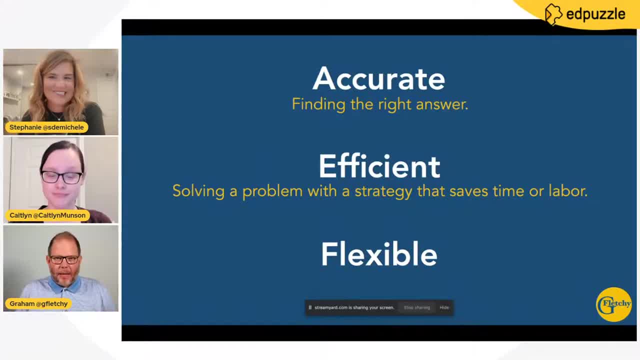 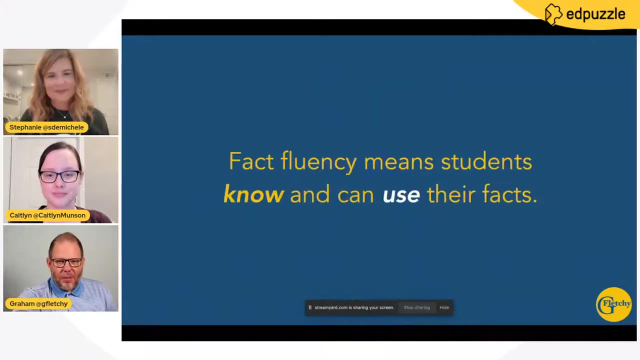 some kind of understanding of a strategy that saves time or labor, Thinking of nine plus nine. do students count on from nine Or can they think of it as, oh, 10 plus 10 minus two, And then flexibly if students can have multiple solution paths? So with that research, that 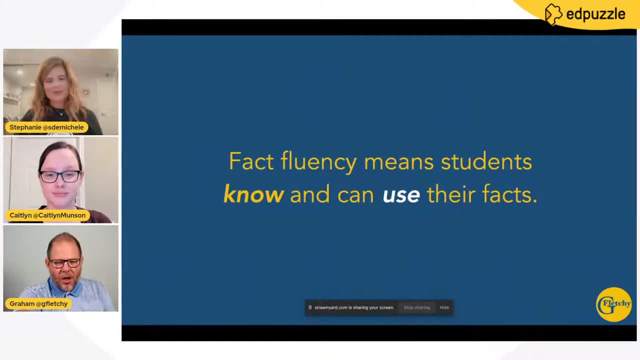 we just shared. the part that was missing for me for so long is that students don't only know their facts, but they know how or where and when to use them. I think about so many of our gifted students, students who can quickly recite the facts, but they don't know how or when or where. 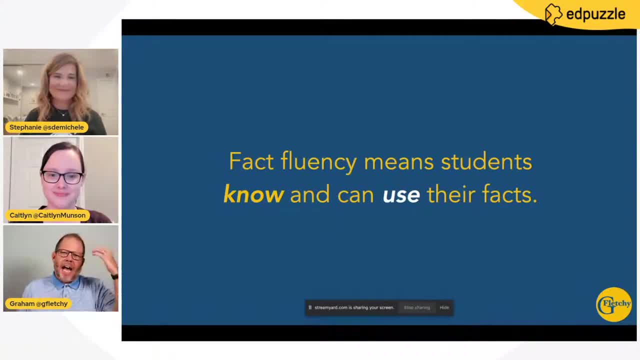 to apply them. For instance, kids would come to us and be like, hey, do I add or subtract this problem? And we're like, no, that's the figuring out part of it, It's not just about the computation. So I want to go back to this research And again, 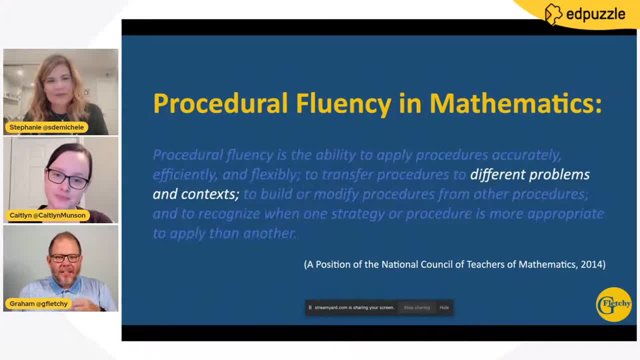 this is where my blind spot was- is that students need to be able to not only have fact fluency, but they need to know to be able to apply it in different problems and different contexts. So what would fluency look like if we started building it through context? So 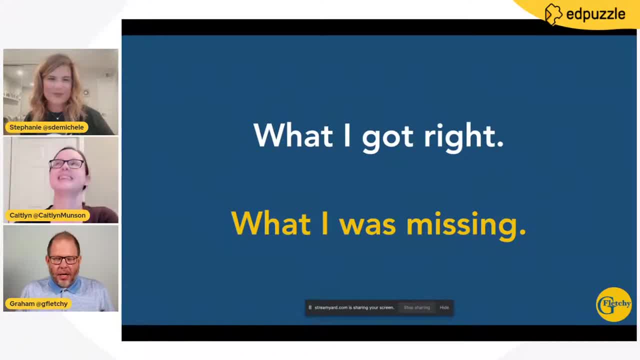 those I've been using number talks. I love number talks but we would be 10 strategy, where kids are adding nine plus seven. Kids could make a 10 during number talks. but the second that we give them a nine and seven in a word problem, they'd revert right back to counting on And I'd be like 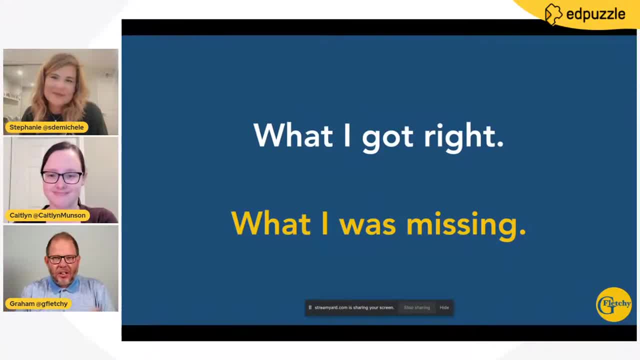 why aren't you using your number talk strategy. So what we're tending to do is we're teaching a lot of strategy. We're doing a way better job today than what we were doing yesterday or the yesteryear or many years before, but we're teaching strategy void of context. Because if we think of 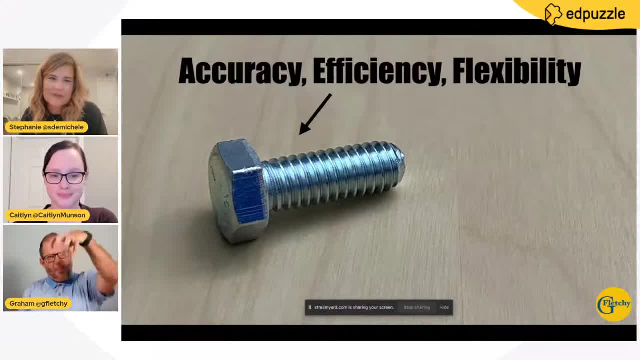 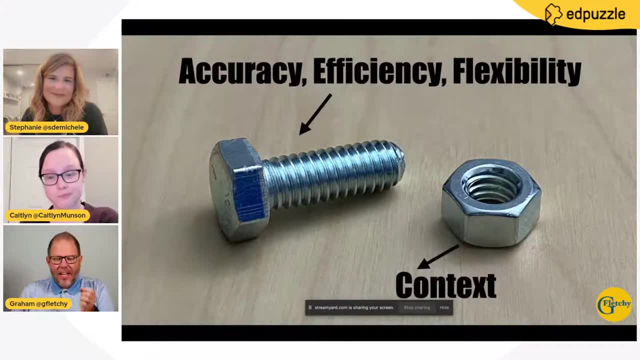 accuracy and efficiency and flexible as this bolt. if I drop this into a piece of wood and I flip it upside down, there's nothing anchoring that. We need the context. It's the context that holds that fluency and gives meaning to that fluency. You can know all the sight words. 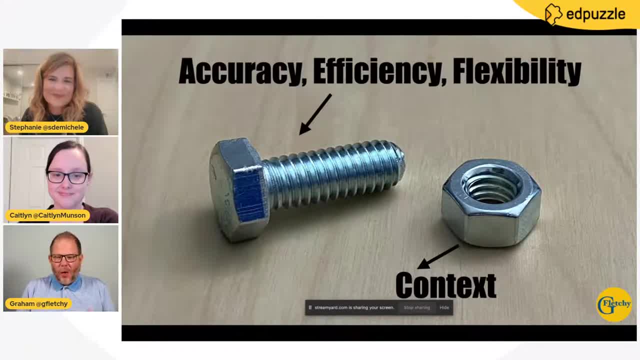 that you want to know, Steph, but the problem is, if you don't know where those sight words fit in appropriately, they're useless, right? So here is where context means so much. So for the next 12 minutes that we're together here, I want to look at what would the nuts and bolts of fluency look? 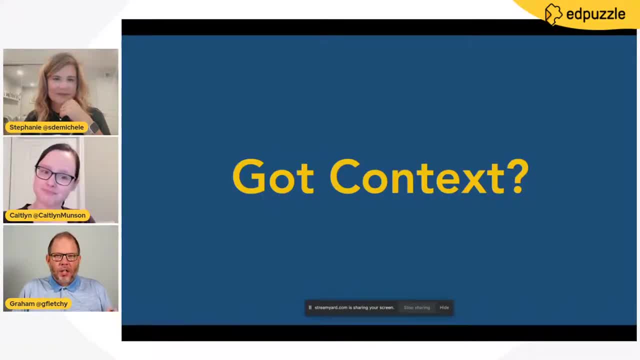 like if we built it through a context. So what we're going to do is we're going to work through a lesson string. So a lesson string is a series of routines and activities that are purposefully connected, that highlight a strategy, but are all built through a singular context. So here's the first one. I'm 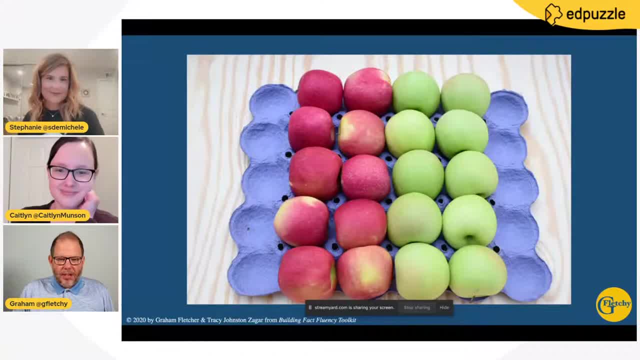 going to be in front of a group of kindergartners and I'm going to show them this image right here and I'm going to ask them: what do you see? How do you see them? How many apples Drop some things. 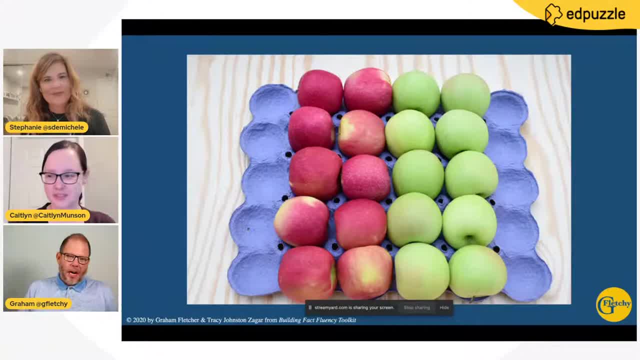 in the chat window, if you can, Caitlin, Steph, as people are asking: how many apples? How do you see them? And before I even saw this, I was going to say Caitlin was yesterday giving me some prep today. 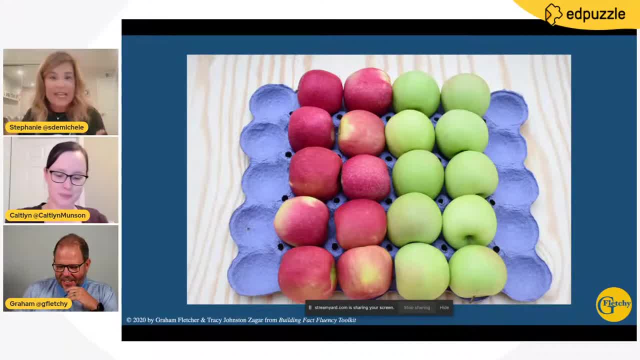 And I was always taught there's a right answer and there's a right way to do it, And so I think that's why I have such math fear, And I love to see this new idea that it's not yes, there's an answer. of course, two plus two always equals four. 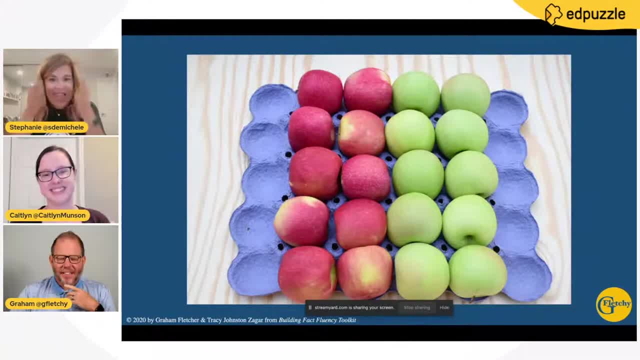 But you know what, How you get there is up to you, And I feel that that is like I want to go back to. I can't go back in time, but I really want to go back in time and be like: why didn't you do this? 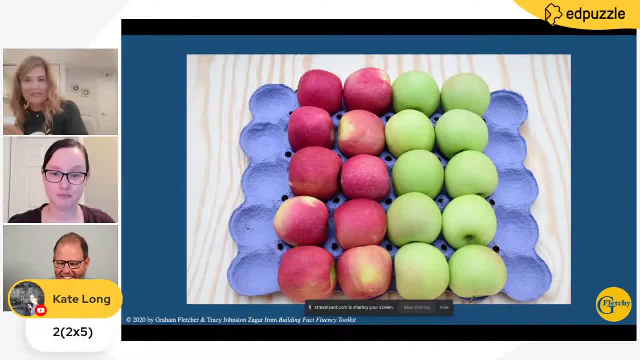 So yeah, I mean, I see columns Caitlin, what do you see? Yeah, so I saw ooh doing some distribution. This is lovely. I saw the two groups of 10. So I could see the block of apples and I guess really for the of each color. 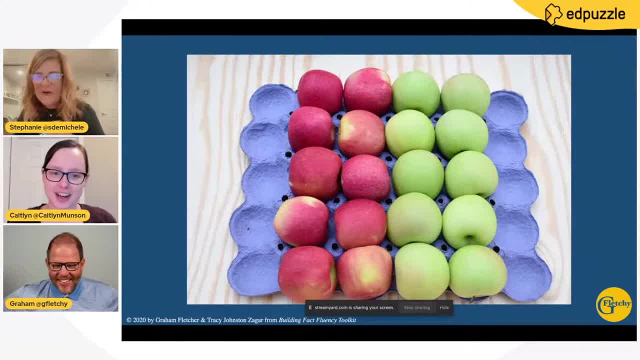 Oh, I'm seeing in the chat, It's just so cool, I get excited. I get so excited about this stuff. Yeah, so I saw two groups of 10, but if I break it down, I don't think that I can, like, at a glance, be like: hmm, that's definitely 10.. 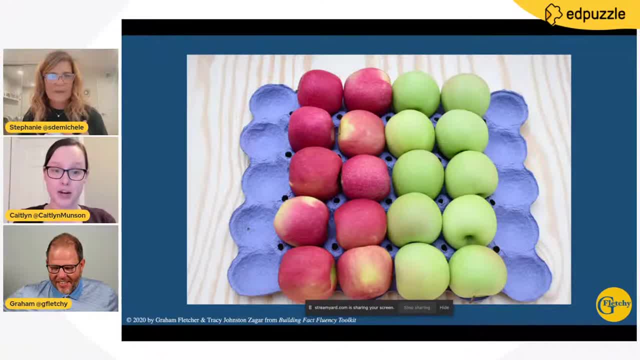 So I think I may have done a quick count of two by five, kind of broken it up into like an area model for each color and done like a two by five to get that 10.. So kind of like Kate, where Kate's seeing two groups of five. 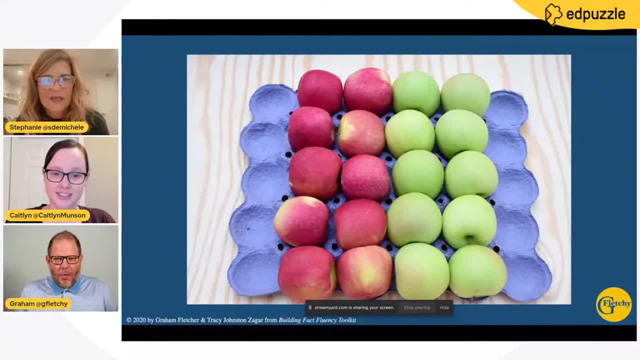 I'll be honest. where, like some of you are looking at this and 10, if you're a primary teacher, 10 frames are screaming at you right now, Like, but here's the thing. Like where in the real world would you ever see a 10 frame? 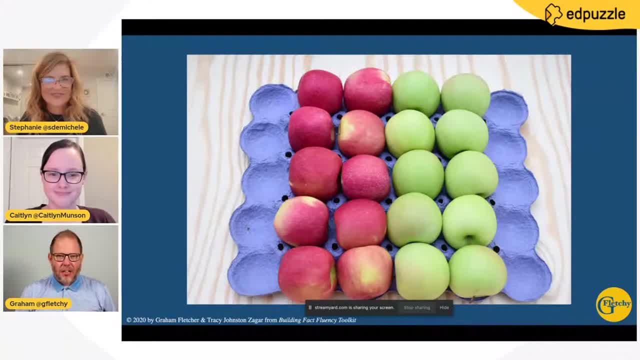 We don't. But a 10 frame is like our Frank's hot sauce, right Like we put that on every single K-2 classroom, but it's out of context, So you'll have students who will count them all by ones. 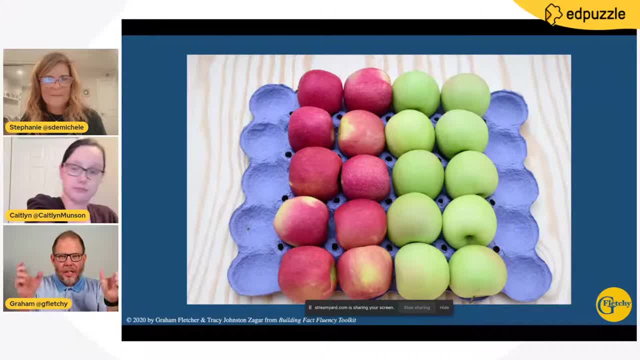 You'll have students who will skip count by fives, Some will skip count by twos, Some will see the double 10.. Some kids will skip count by fours- four, eight, nine, 10,, 11,, 12,, 13,, 14, because skip counting by fours kind of suck and it's hard. 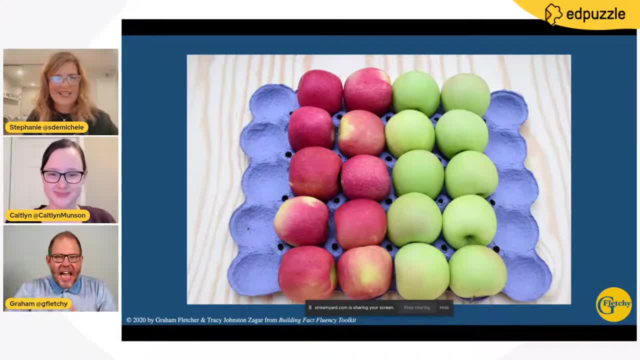 And so they might not be able to do that piece. But here's the thing. Next image: So here's that. in that image string, in that image talk. the images are connected. Now, how many couples are there and how do you know? 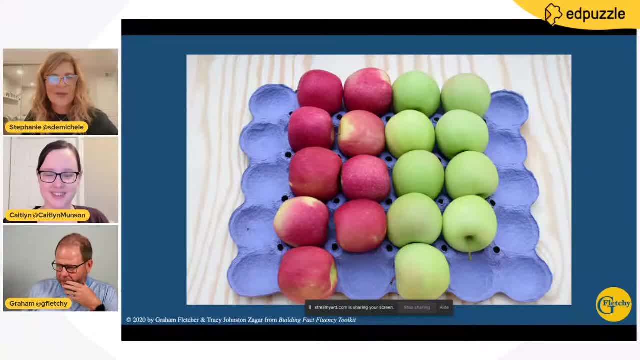 Oh man, Can you move to that window please? Wow, 30 minus 10.. So, Joe, what you're seeing there is: you're seeing the whole tray holds 30, but you can see the two columns of five. 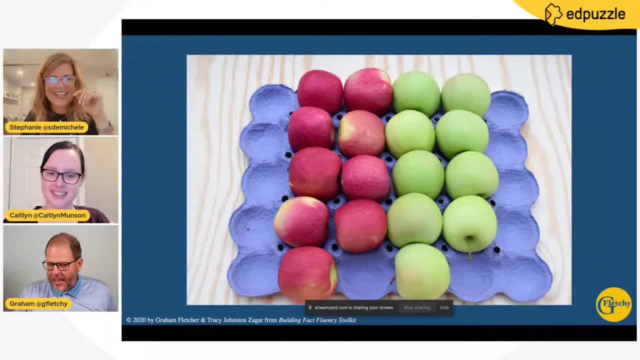 So it's five. 10 are missing from the 30.. Awesome, Nice, Some students kindergarten class first, second, third, fourth- I'm going to look at this. I'm going to be like, well, we just had 20.. 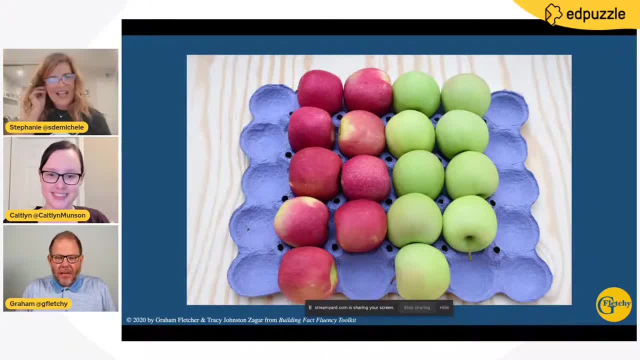 We took two away, Now we have 18.. Some kids will look at this and be like: oh, I see nine, and nine is 18.. Some kids will say: well, I see two groups of eight, That's six, Four left. 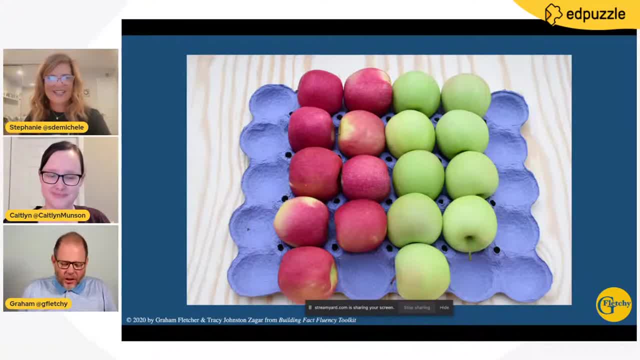 I was in a first grade class and a little lady says, Mr Fletcher, she goes, I didn't use doubles like everybody else. She says I closed my eyes and I picked up that green apple and I just rolled it over and I pretended that I had 10 red and eight green. 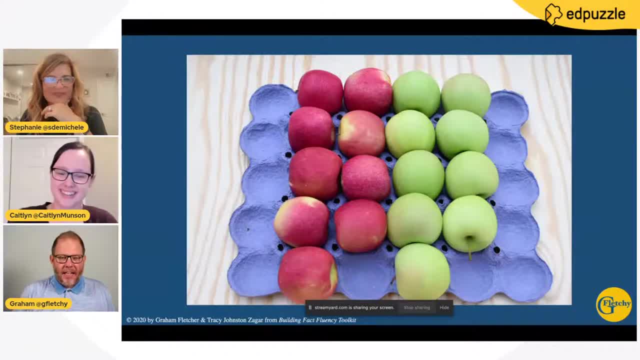 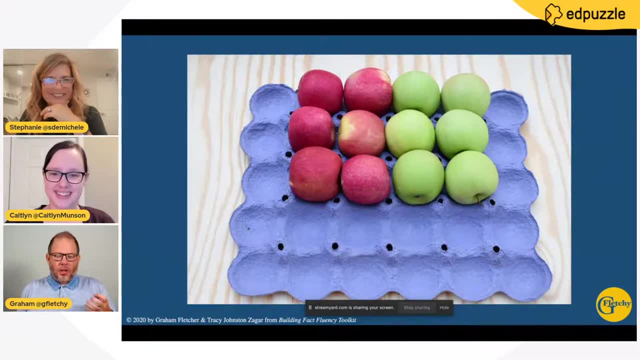 So you've got the associative property. there We're making a A 10. There's the next image and the next image. So now you can see that we're talking about this idea of doubles. That's our strategy. But the context where the numbers are now ingrained in a context, the context is apples. 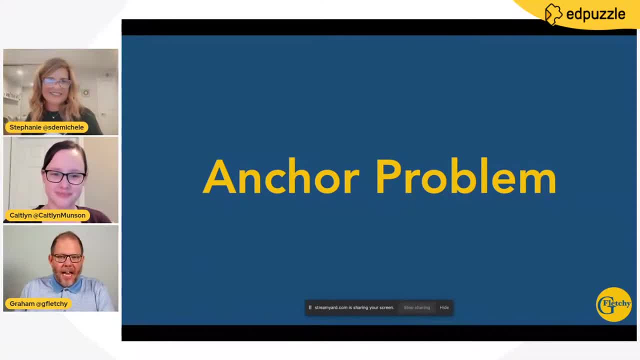 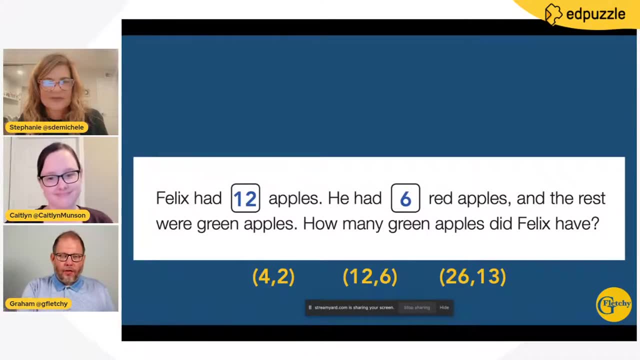 So next we follow up that image talk with a anchor problem, And all an anchor problem is is a word problem. Here you can see just some number choices on the bottom. Those of you who are familiar with cognitively guided instruction, CGI. 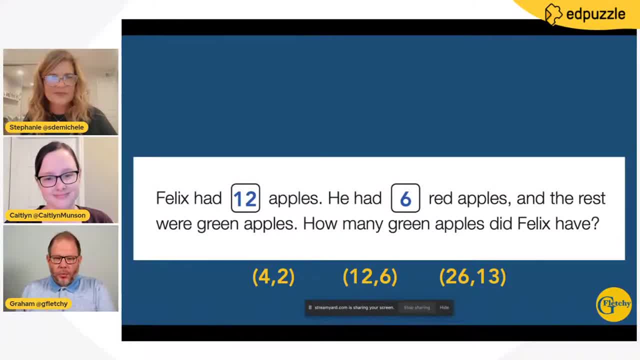 but Felix had 12 apples. He had six red apples and the rest were green. How many green apples did Felix have? Well, you know as well as I do it doesn't matter the grade level. When kids look at a word problem, the first thing they say is: oh, that's too hard. 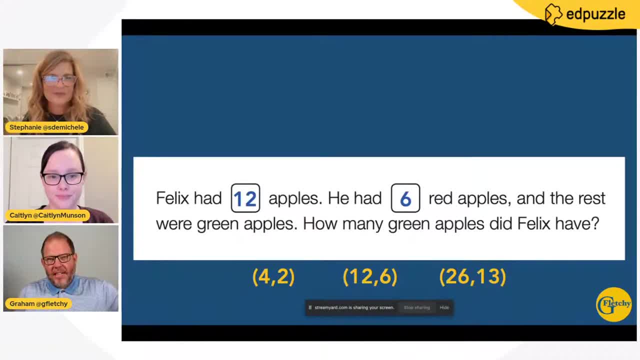 I can't read it. What ends up happening is because kids now have an image of apples and an understanding of context and meaning that they can bring to the forefront when they tackle this problem. it's much more accessible for many of our students who struggle with the language. 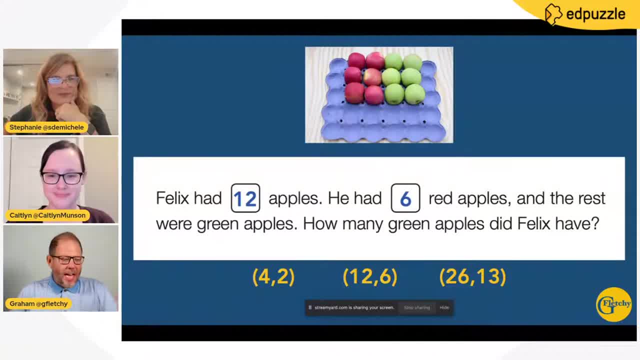 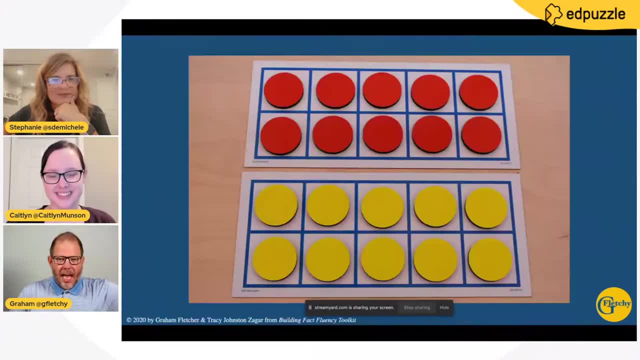 around the mathematics That we're trying to learn. So there we have the image, talk and anchor problem, And now what we do is we start to strip away the context of the apples and we replace it with a tool, And now we go ahead, Steph. 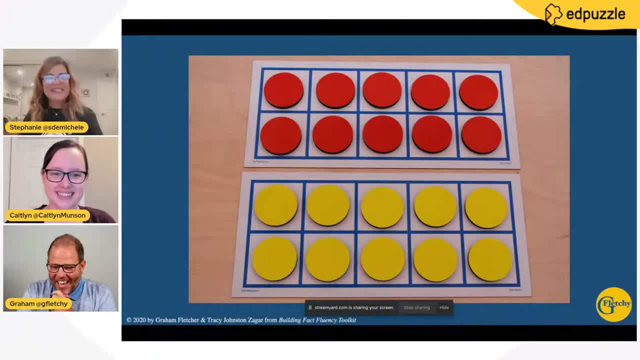 Now, no, I got to jump in, So it's OK. So I was. I was an English. I was the only teacher I taught high school. So I always would say: a picture is worth a thousand words, So don't just cruise through the reading. 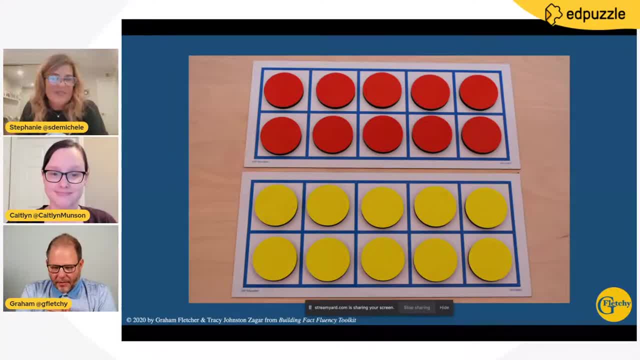 Look at what the picture has to say. And so now I'm seeing it applied to math And I'm like I got goosebumps. I'm like, yeah, yes, the image is important in math. So, yeah, media and video are where our students play like they have a lot. 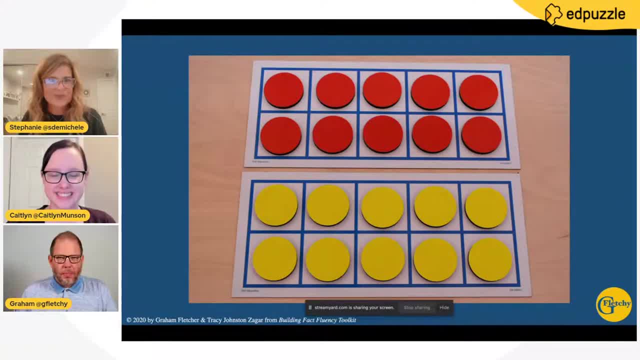 of space there, whether we agree with it or not. We'll save that for for other people to kind of argue with. But I think, as teachers, how is it that we can leverage media? How can we leverage video to to bring more understanding, to create more accessible? 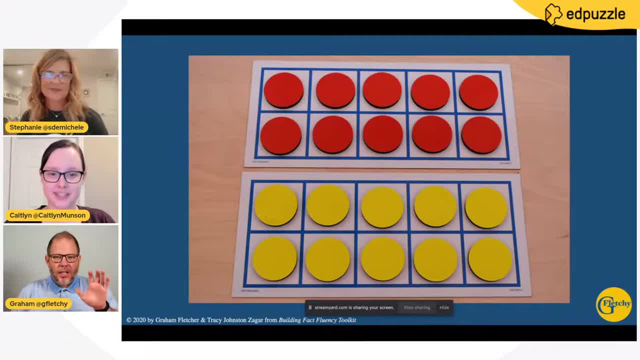 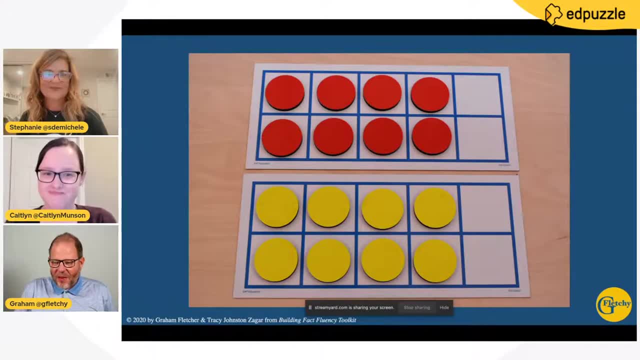 mathematics to where all students can now tackle this problem, Because when students are looking at the 10 frame, they're also picturing those apples that they just saw. So I think that's a really big piece that you're talking about there, Steph. 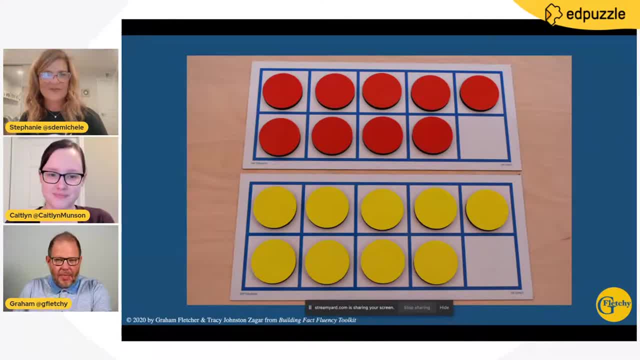 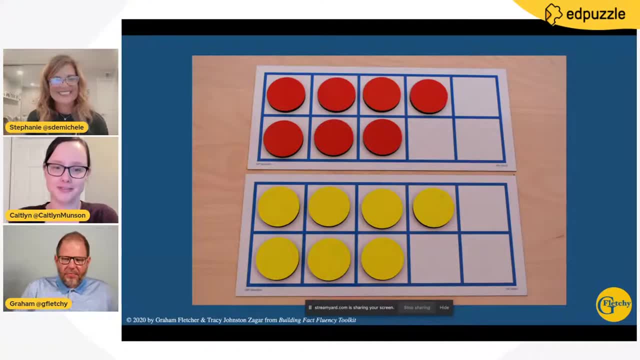 is, is the the connection between language, image and, again, just trying to make it accessible. for sure, Yeah, Building that bridge as we go from the concrete of apples that you can like that little girl who rolled the green one over to be with the red. 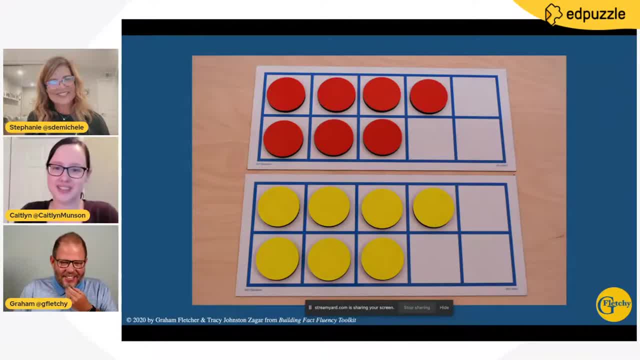 the concrete to the very abstract. This is beautiful. It really connects the manipulatives that students hopefully are getting to do hands on with, which are concrete, yes, but tying it back to something with context, So it's not just red dots of yellow dots. 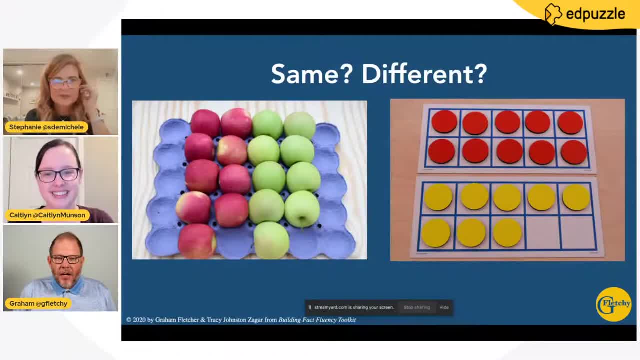 Absolutely. And then this continues then. And so now you ask: like, what's the same, What's different? Like you see, So we're being really intentional about what's called contextualizing, playing with math in a context and decontextualizing it, taking it out of of. 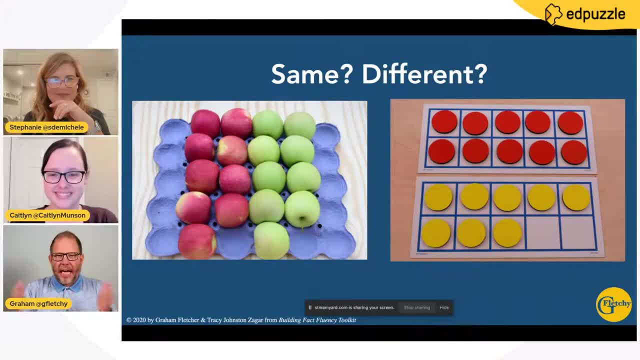 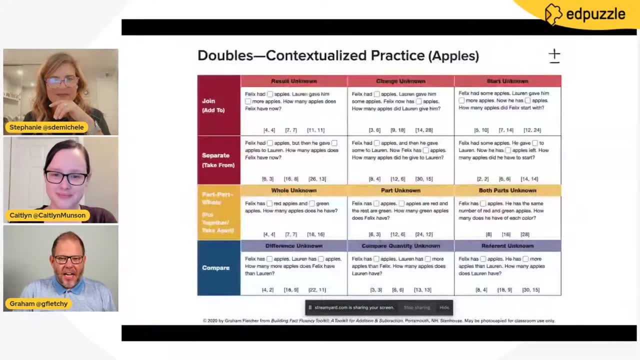 of the context and playing around with just counters, counters that have no meaning. But if we want to apply it to an understanding of apples, we can definitely do that piece. And then here we'd follow it up with with some all the the problem types that many of our students would need to play around. 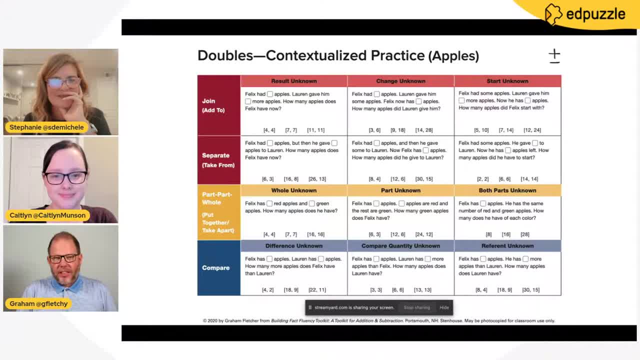 with start change. result unknown. all of the problems that you see here are all grounded in the double strategy and they're all around the the context of apples. And then next is: you can see how we've done an image talk, an anchor problem. 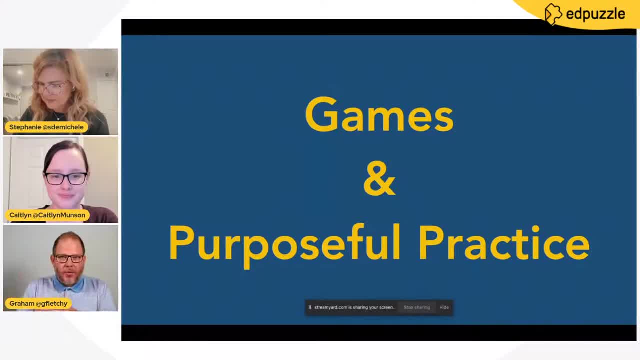 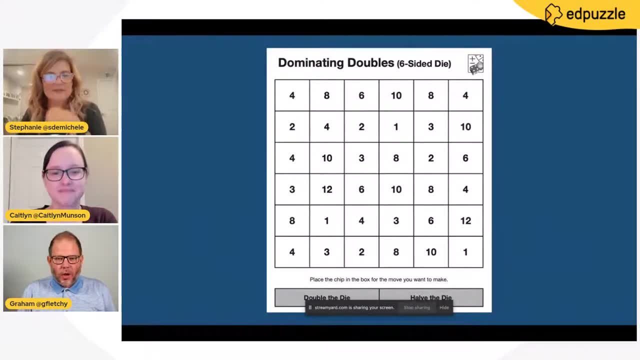 like a word problem, Then we did the tool talk, Then we play around with some of those other problems And now we have a game And most of the time our games are basically dice generated worksheets and they're not engaging for students. 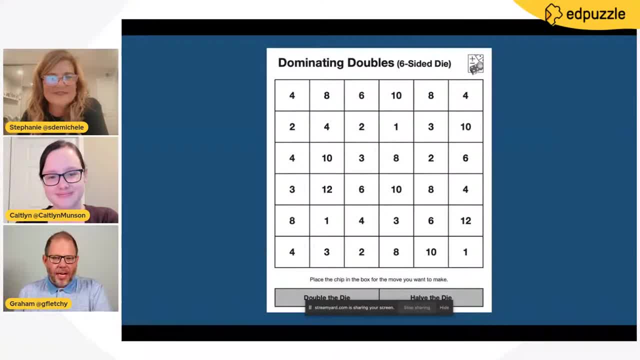 But here students roll a die, And when they roll their die they can either double it or they can half it. So there's a student choice there again, giving student autonomy, just trying to play, connect for, but playing with that doubles and having strategy. 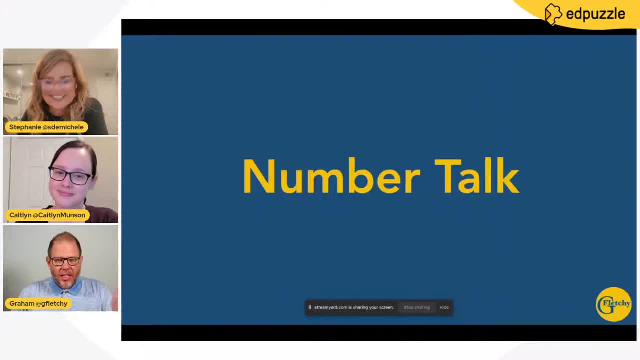 And then, at the very, very end here, as we've walked through this lesson string, or through this lesson string, we now get to the number talk, the naked numbers. So when kids are seeing two plus two, three plus three, four plus four, they're not. 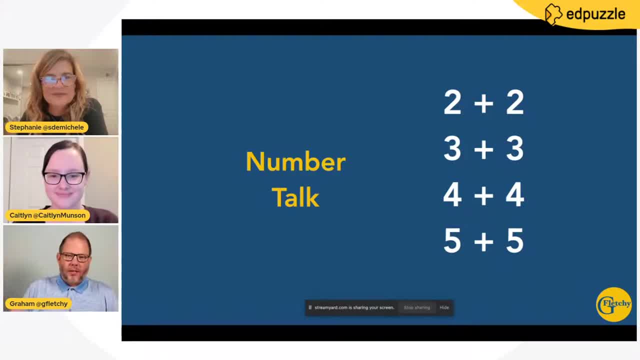 just seeing naked numbers. they're really seeing two red, two green, four red, four green, and it's about giving meaning to symbols and numerals, And too often that's what we've been missing for for for for quite some time. 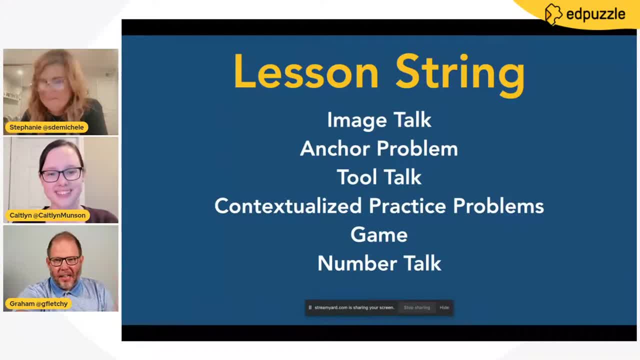 So what I want to kind of share is that's kind of how we've kind of worked in. there's the mathematical arc, mathematical storytelling. we've talked about apples, And as we've talked about apples, we've embedded this idea of doubles, so we can 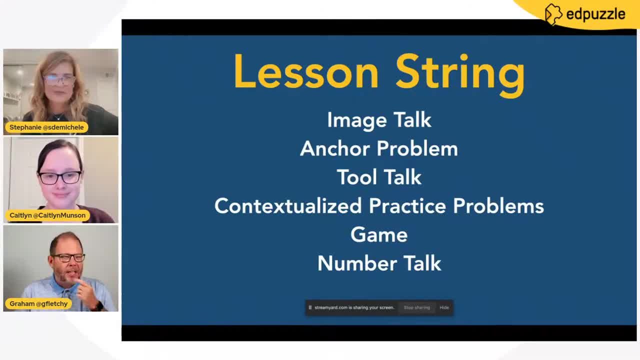 come back. kids aren't going to remember a double strategy, but we can come back. Remember when we shared those pictures of apples and there was the same number of each color. What's that called? And it's because of the images that we've. 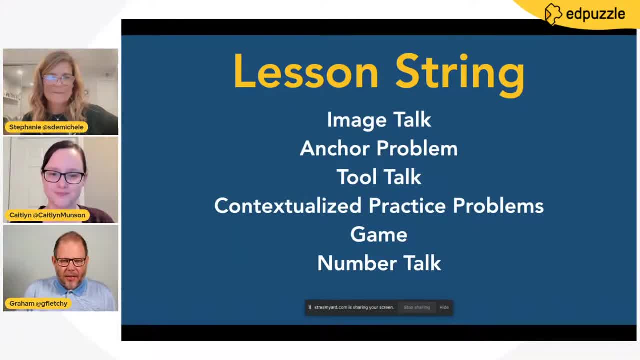 built and left what's called a mathematical residue- things that stick kids. So does this replace like drilling, like when I had to Drill with flashcards? Does this sort of replace it? Yeah, heck, yeah. So I think about like my like, where I think many of us were all given flashcards. 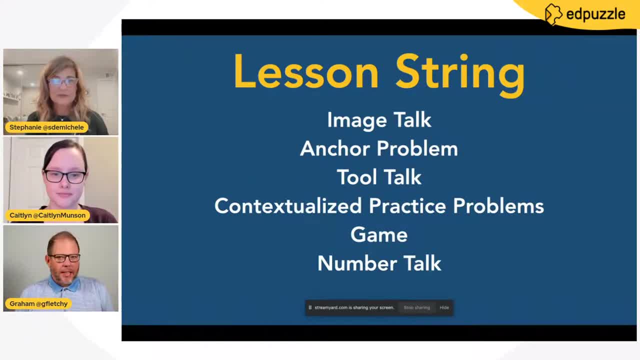 And if you don't couldn't memorize your facts, what would people say Like memorize harder, Yeah, you need to be punished. It's like writing at the board, except it's writing it on paper. Gosh, I remember having to write them and just repetitive repetition. 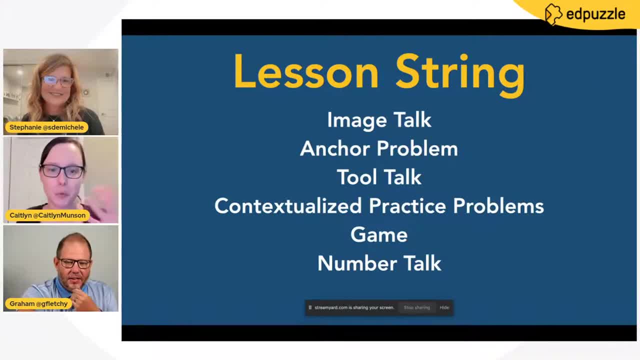 Like after a while the numbers don't look like numbers anymore. It's like when you say a word enough times, it stops sounding like a word, it completely loses meaning: Absolutely, Absolutely. So I think I think for me it's about it's. 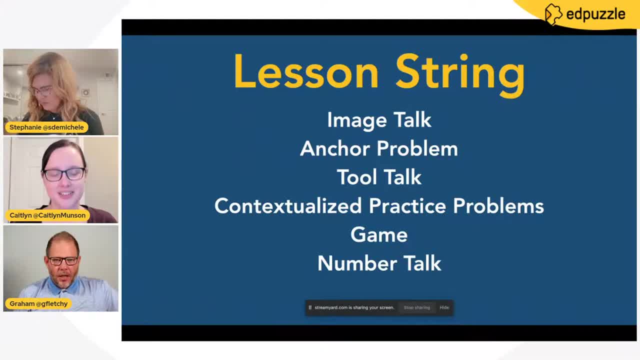 making sure that fact fluency is an outcome of problem solving. It's not a precursor, it's not a gatekeeper to problem solving. But for too often we've said: if you don't know your facts, you can't tackle the big boy math. 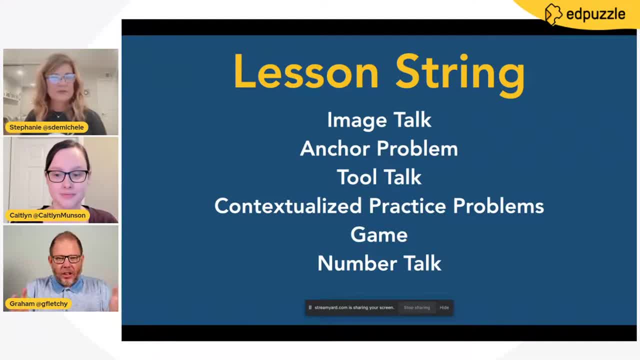 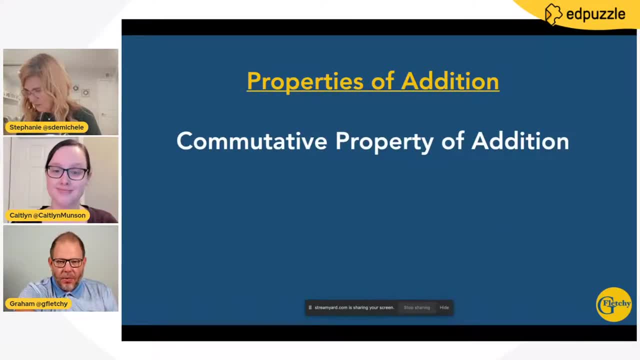 But really there's a lot of understandings that need to go ahead and need to take place. So here's kind of what we're sharing Right. So like right here, this little session that we've done. here we've talked about the commutative. 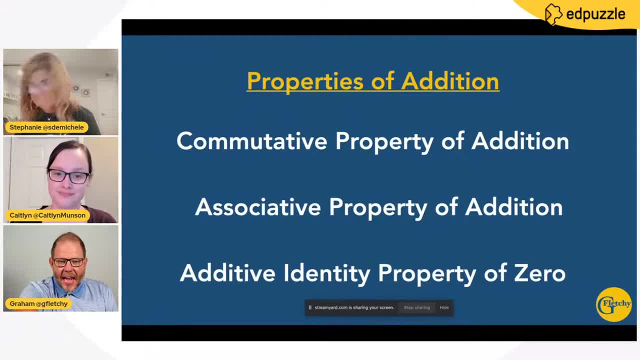 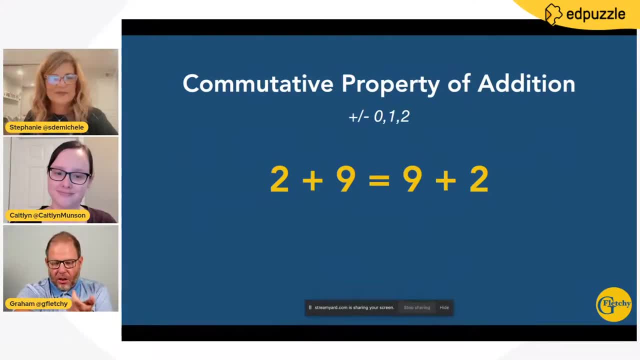 property, associative property, where we're making a ten, and the additive identity property of zero, where we use the commutative property. when we add two plus nine- but maybe we start at nine plus two, We can switch them around. It's about that: relationships, that's scalable. 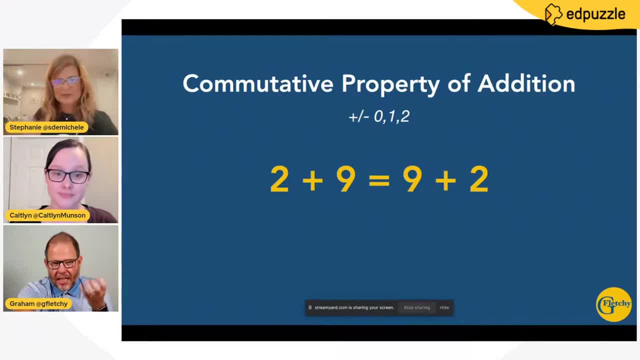 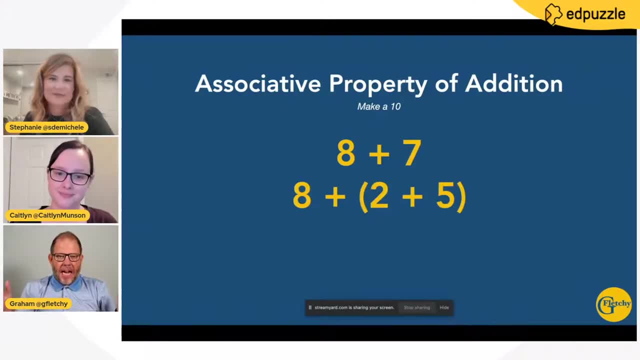 So, like Caitlin, you in middle school, having teaching middle school, making sure that kids know these properties, the associative property- when you make a ten with the associative property states, is that when you have three add ins you can actually group the add ins. 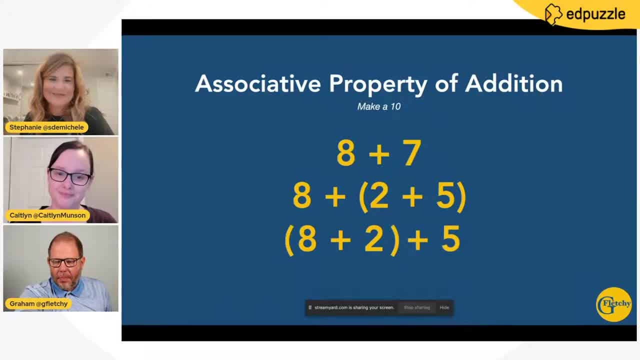 However you'd like, and you'd still get the same sum. So here, what you're doing is you're associating two from the seven with the eight to make a ten, And that's how you get ten, Fifteen, That's how you get ten plus five is 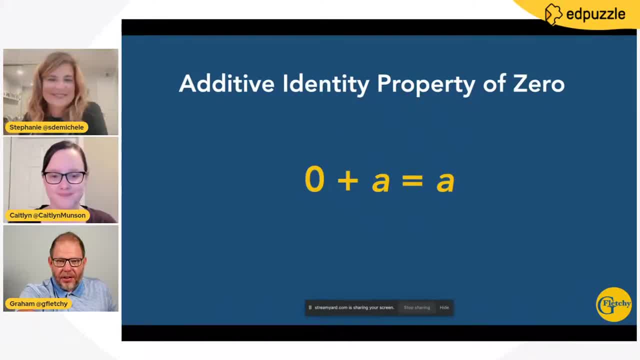 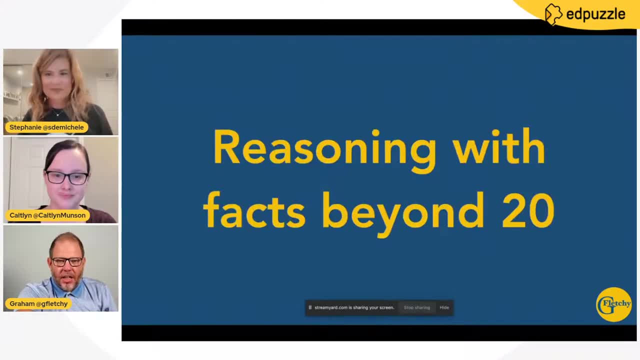 fifteen, and then the additive identity property of zero. So I know that we've talked just about addition and subtraction here, But but what I want to do here is just make a quick connection. It's about not only just knowing your facts, it's about reasoning for years to come. 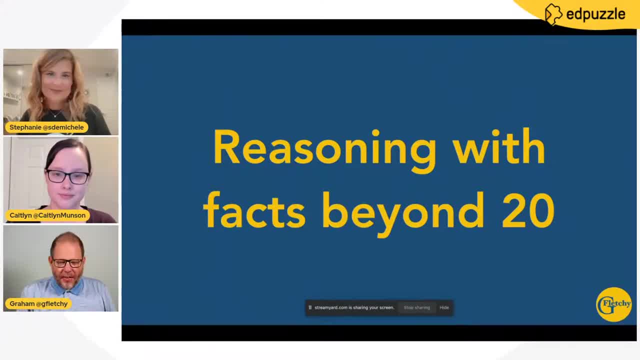 I know this is one of the questions that we are going to tackle, like: where does abstract fluency fit? Well, it fits into every grade level, But it's not just about knowing your facts, It's about understanding the relationships. So here's where what we're learning. 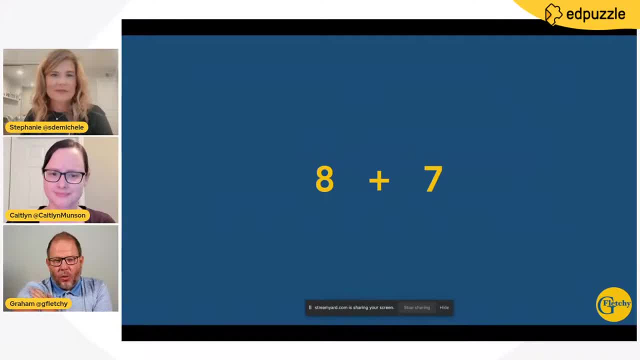 in kindergarten is scalable through fifth grade and beyond. We use that associative property when adding eight plus seven. take two from the seven, give it to the eight. Well, it happens when we get into first and second grade and we're adding two digit plus one digit. 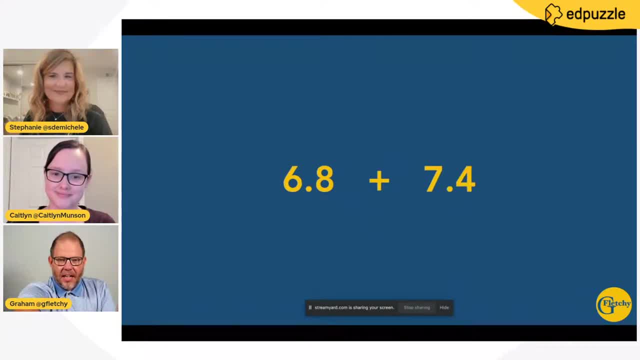 Take two from the seven, give it to the sixty, eight to make seventy. And now, when we have decimals, we use that exact same associative property, where we can move them around and associate different parts of the whole until we can make a sum. Steph, do you want to take a? take a little chance at this. 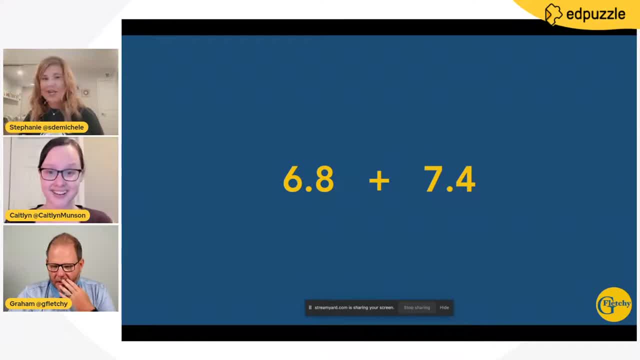 Caitlin, how using the associate OK, OK, So, and it's funny because I've worked out a way over the years for myself to do it just any way I want. I just knew it would work. probably not the proper way. 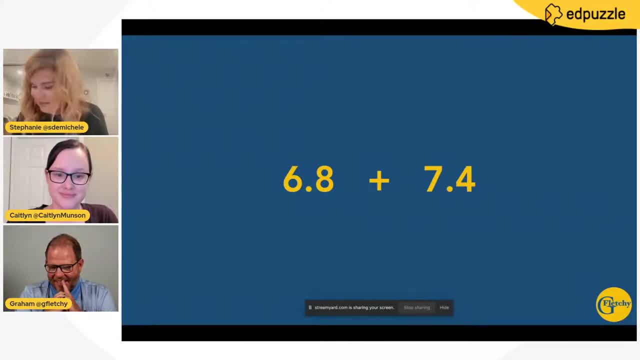 But I always take. This is how I do it: Sixty seven is thirteen, And then I take the eight or and it's twelve, So thirteen is twenty five. OK, that's not right. Oh, I'm wrong. I know what you did, though, and I know it's tough, because you said: 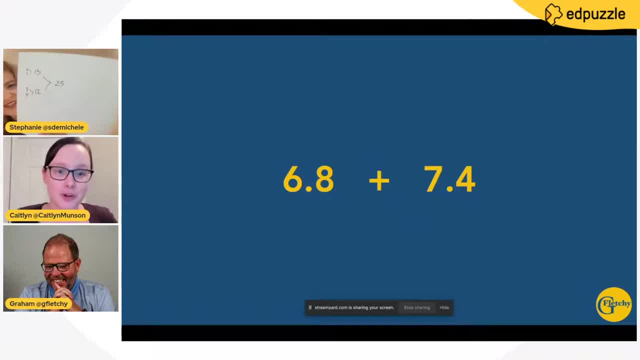 you're. you're reasoning out loud, which is beautiful, OK. so when you did your eight and your four, is that really an eight? Oh, oh, OK. I see what I did. I see what I did, Like, hold on. 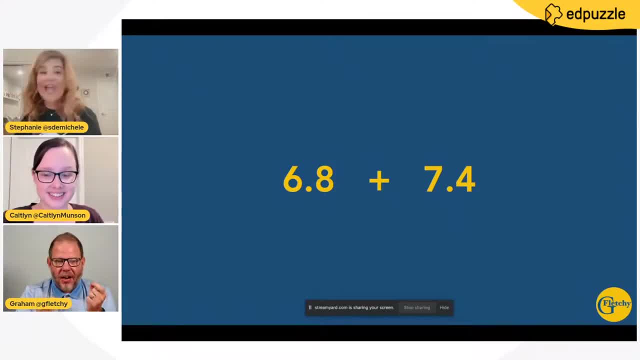 And in the chat window, just as Steph is thinking through her thinking: Yeah, you'll have plenty of time. No, you're great, Keep working, Keep working. in the chat window, How can you use the associative property to find the sum of these two add ins? 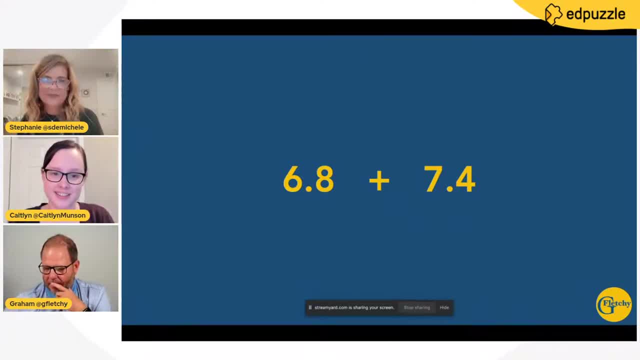 Maybe drop something in the chat window as Steph is finishing up her thinking. So another way to think of it, Steph, would be: how can we make that six point eight a friendlier number? What can I borrow from seven point four to make six point eight? be a nice friendly. 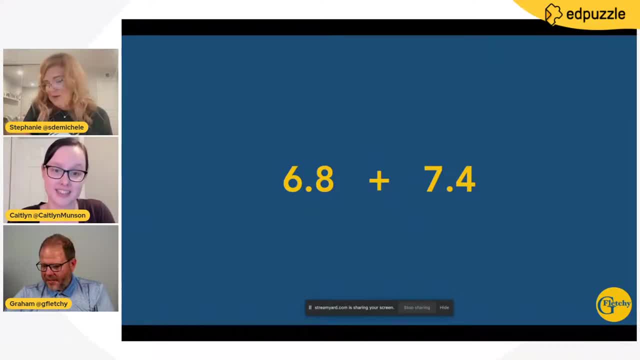 number. I'm going to make seven point oh, and then seven point two. Right, Yeah, that's it. So you're taking two tenths from the seven and four tenths giving it to make a whole. There you go, Perfect. 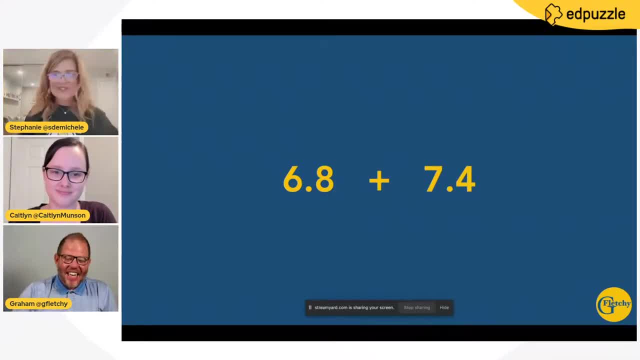 Nice. And then this, the same understanding. it happens with multiplication as well, to where, when we're building our multiplication facts, when we're building, when we're building multiplication, we're using the distributive property, and that distributive property goes all the way up into high school when we talk about quadratics, where 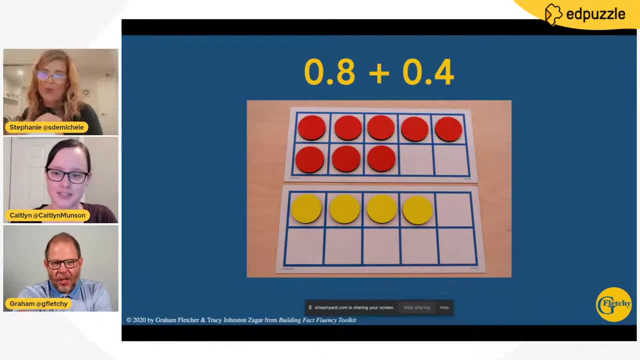 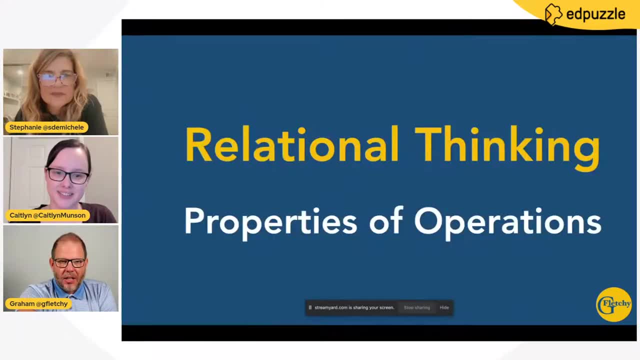 And so here I can, actually I'll give you a quick example, just another, just example here, of using ten frames again in in fifth grade with your grade five students, where the ten frame is the whole. But here's just the example. Caitlin, I threw this in here, knowing you working with middle school. 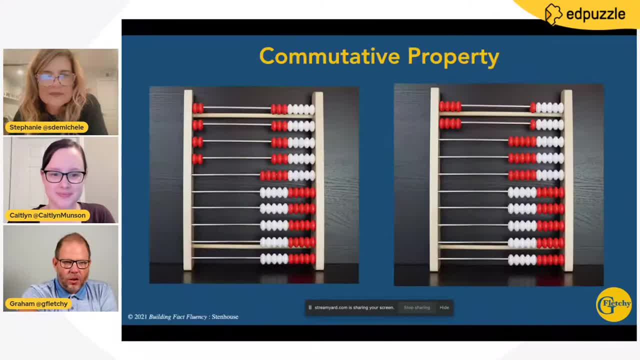 In high school. I also noticed that that Kate teaches high school as well, So she uses money. she said Yeah. So here you can look at the commutative property, where you've got four groups of two or two groups of four. 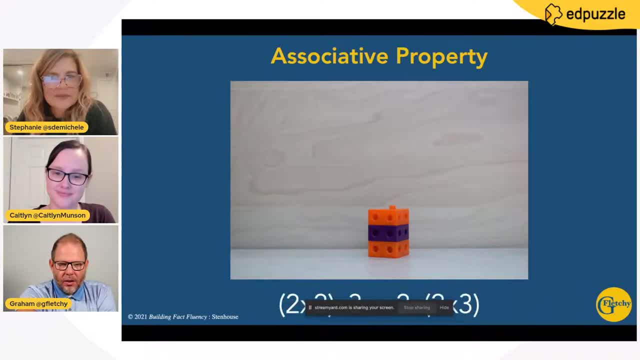 You also have the associative property. How many cubes are here? Well, you could say two times two for the base, times three. Or you could look at it in terms of layers. You look at it as slices two times three, and then you double your your slices going. 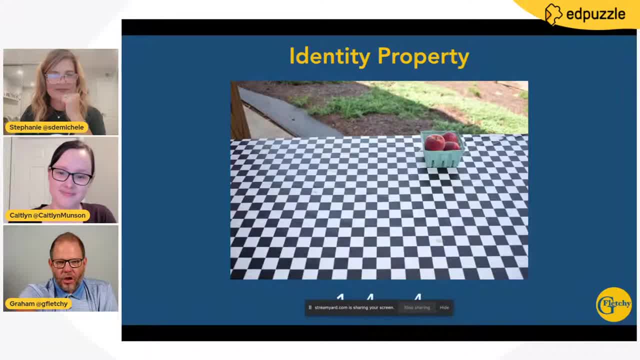 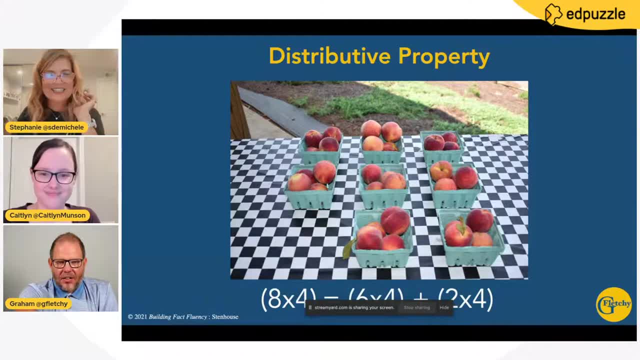 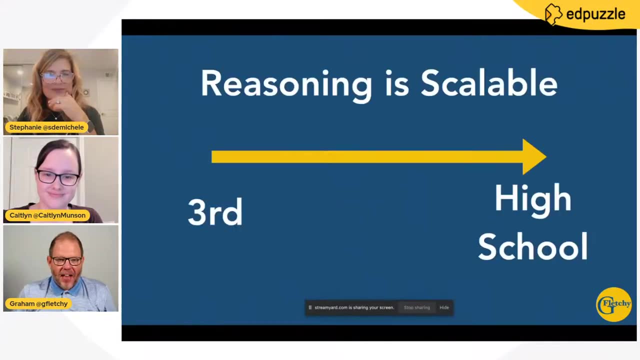 vertically. Then you have the identity of one group of four is four, and then eight times four. Well, you might not know eight times four, but you might see it as six groups of four up in the top plus two groups of four at the bottom. So here's the scalability of that thinking. 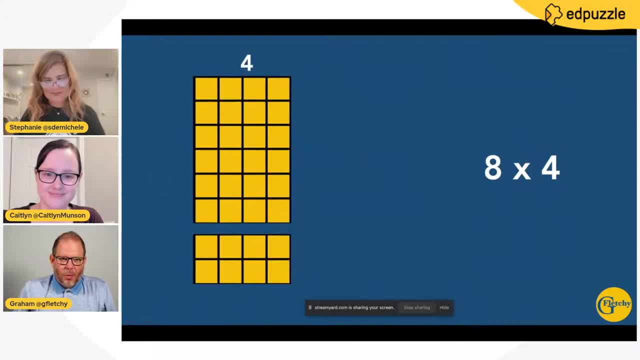 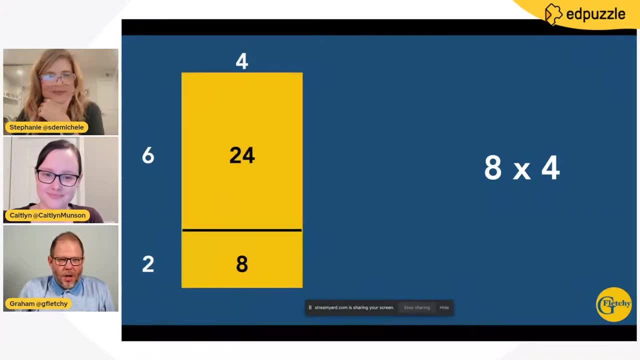 Well, in third grade it goes all the way to high school. Eight times four. We're building arrays. This is third grade. This is what we do. It's eight times four is the same as six times four plus two times for open array. 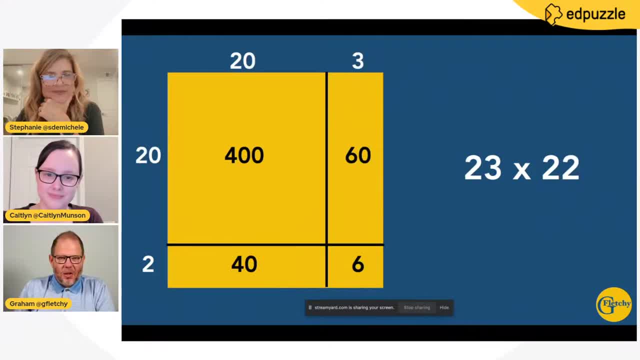 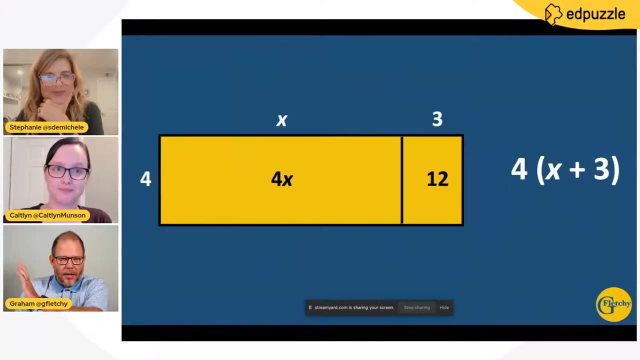 model. Then when we get into fourth grade we use two by two digit multiplication, partial products, distributive property. Still it goes into multiplying mixed numbers with fractions. The model hasn't changed The relationship of how we really build true fact. fluency is now scalable. 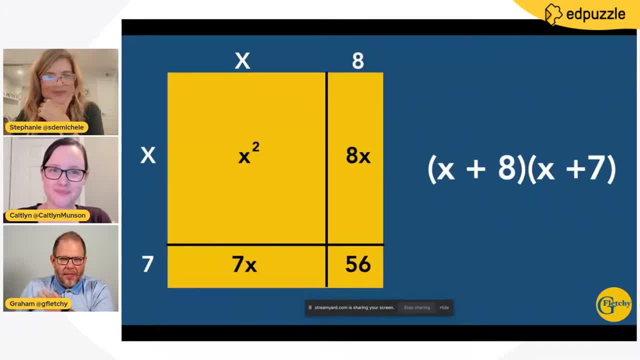 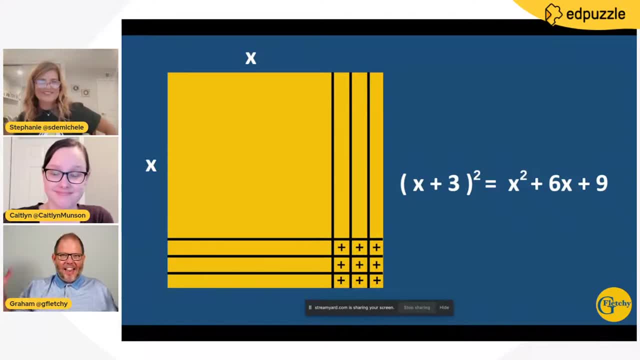 Factoring in middle school, in grade six, seven and eight, and then all the way into high school with quadratics and completing the square. So that is how we can build fact fluency and the same idea. we build that whole story up with multiplication and division. 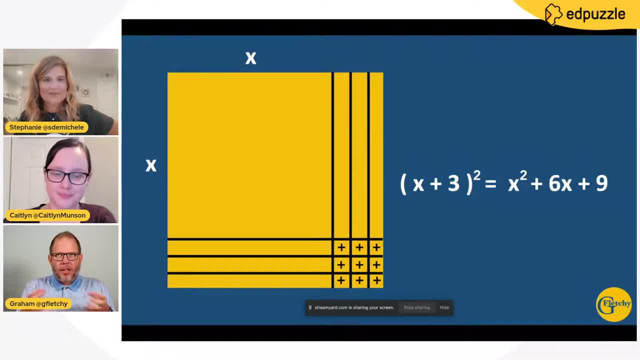 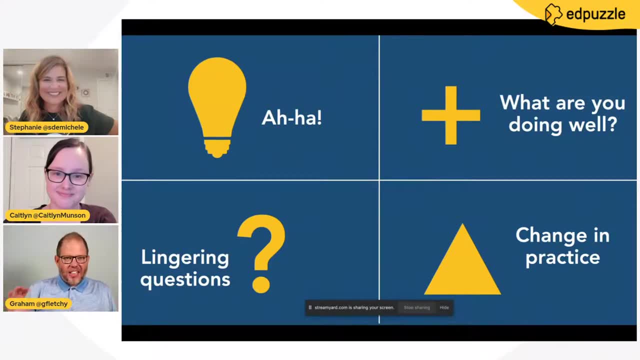 But again, just thinking about, when you build fact fluency, do you build it out of context or are we building fact fluency with just naked numbers? So I know we've got about six, six and a half minutes here. left for, left for. 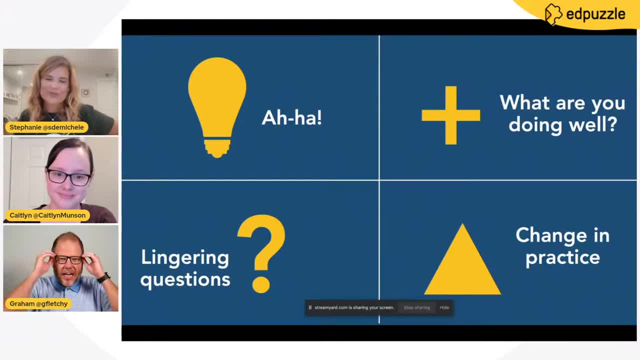 questions, but that's kind of it in a nutshell. So I don't. I'm going to kind of stop talking here for a minute and see, see, what questions you all might have in that space. I'm going to go ahead and stop sharing. 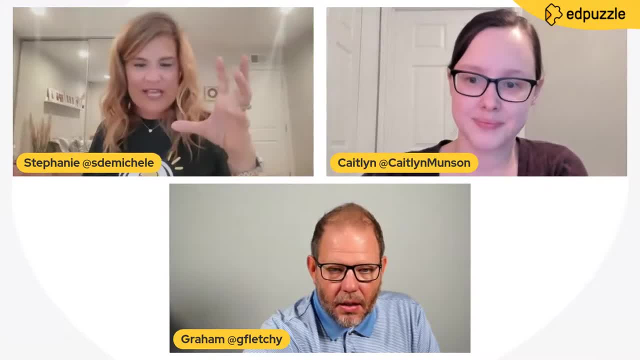 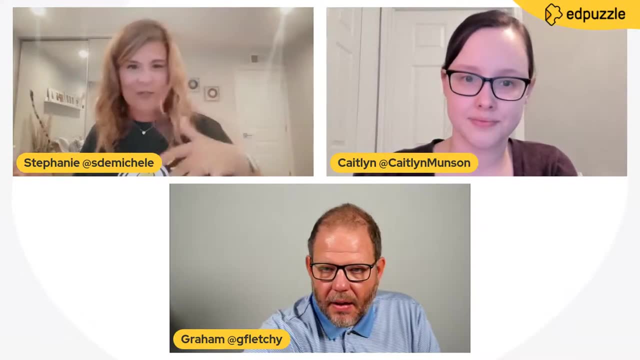 Actually, Graham, could you go back to sharing and put up that slide you had? I'd love our audience to be able to see it where. it was the plan, It was the, it was the image, the anchor, the game, the number talk. 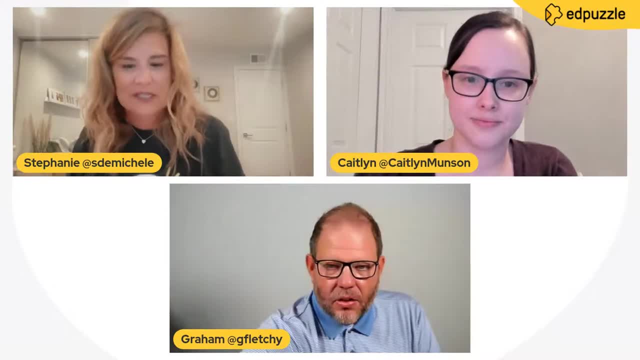 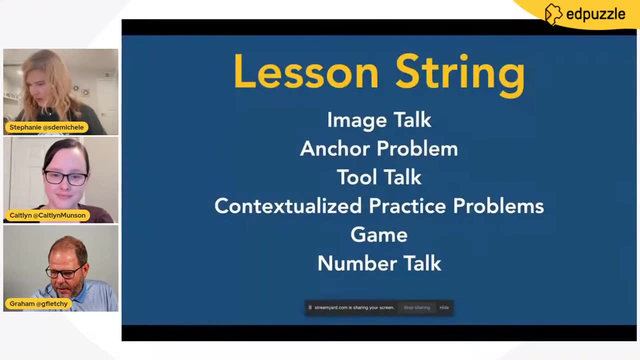 If you would put that slide up for our audience, I think that would be super, like the lesson string. Yes, Lesson string, Thank you. Yeah, I think I got it right here. Yes, that, thank you. And what I can do, Steph, is I can share. I'll share some resources with you. 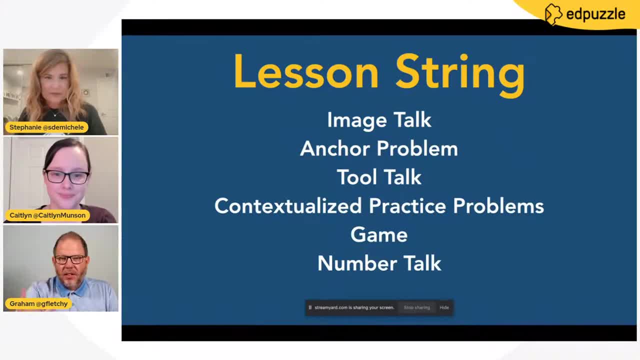 and the team, so when we share with friends, they can actually find places where they can find some of these online. Sure, We have. we have resources to share. Many are. if you're a Marvel fan and you'll get this reference, Manny is our man in the chair. he's not, so he's got all the links to drop for us. 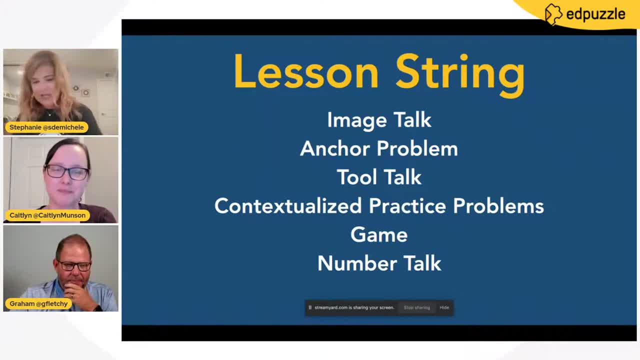 to get more information from Graham and to go to his website and all of that. So if you do have questions, please, please, don't be shy and add them in the chat. One of the questions I had that you answered Graham was, like you know, is this: could this be for any grade? 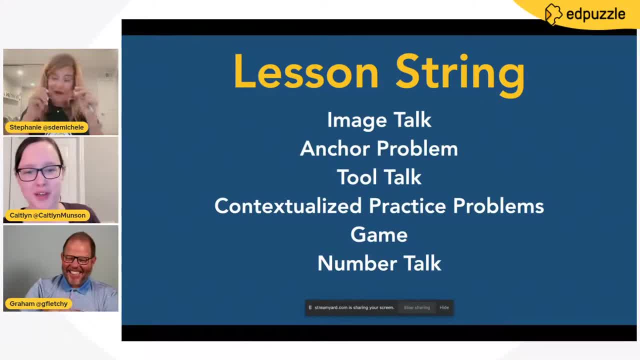 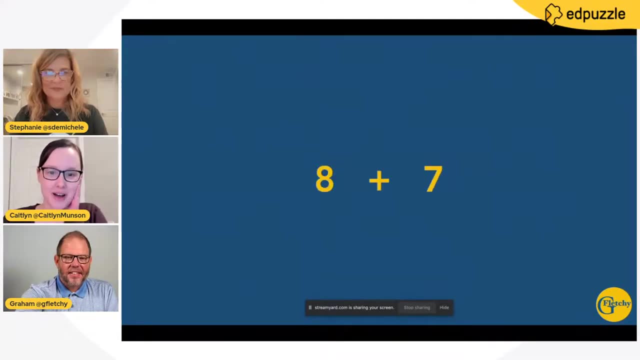 Yes, I can't. You know, most recent years in the classroom I taught algebra one. And yes, absolutely Actually, if you go back to when you were talking about quadratics and but even when you were talking about, like, associative property and things like that. 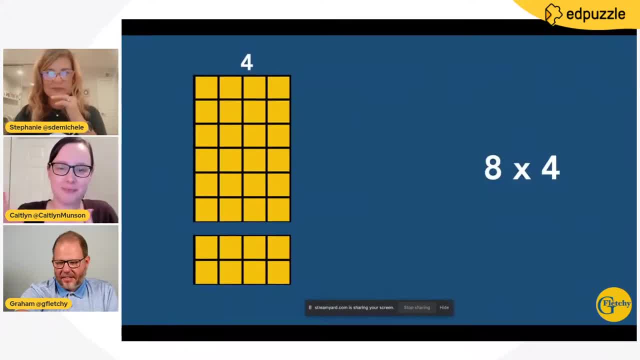 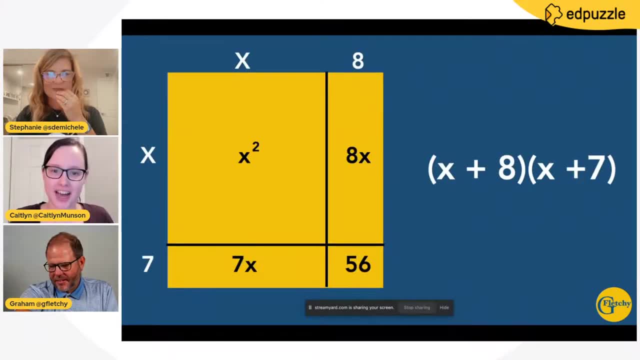 when we want kids to like Solve an algebraic equation, solve for X, they have to come up with a strategy for how to do stuff and they have to be able to play with numbers And find those friendly numbers and building in practice the exact kind of practice you're talking about. 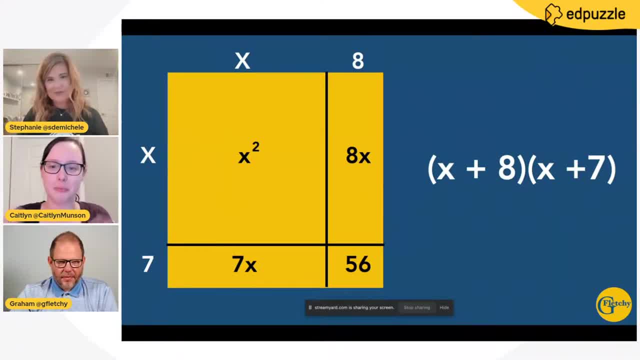 It. yeah, it builds that fact fluency and also bridges that hey, we're doing something that's super abstract and it can be hard to think about it and tie it back to something real. I think this is beautiful. I love the image, the ability to be able to say: Kate, it was kind of like that. 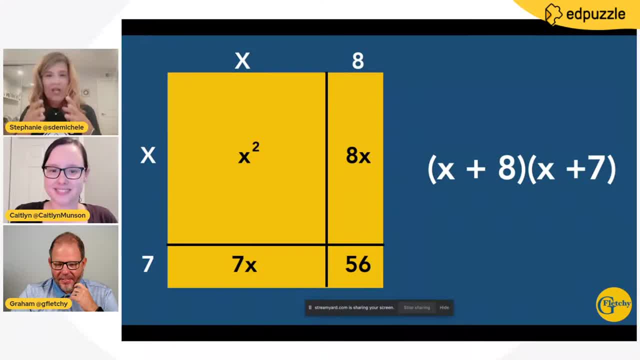 open middle. is that what we're talking about? that there's something that you can do it your way, And I was. it was like you have a formula, you do the formula or you memorize And it's, and so I guess- and that's probably why I always had trouble learning the language and why I 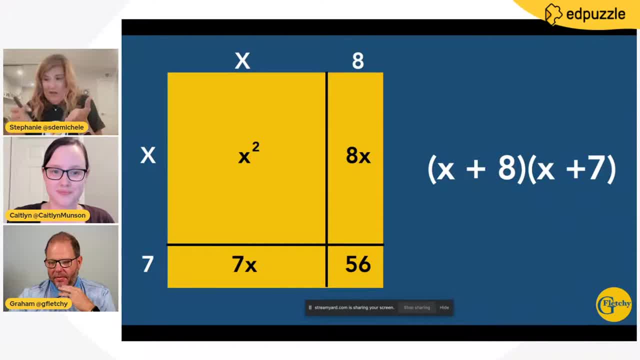 like Duolingo is so much better, because it's not necessarily about how am I going to conjugate this verb, as I'm trying to learn the language It's, you know, picturing something in your head, Right, Yeah, For me. I also start thinking about so many of our multilingual students. 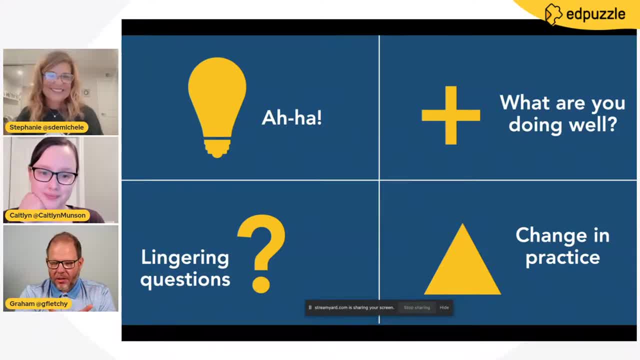 Right, Like they don't have an opportunity because of the images And so they're grappling with both language and the mathematics simultaneously. So, in terms of a of a building, an equitable classroom and an equitable space to where all students can kind of feel like we want all students to feel invited to the math conversation. 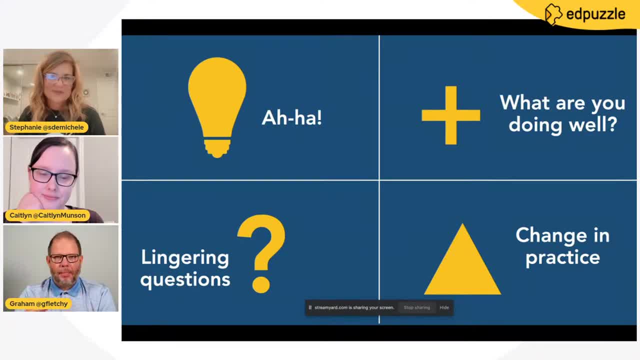 images and media and technology really can kind of begin to amplify those voices which typically aren't heard in our classrooms. Which I think, leads us to a natural question: Hey Graham, In what ways can we leverage video to support fact fluency? 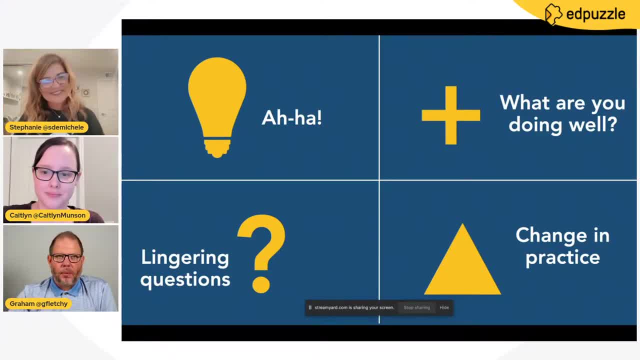 I think this, this is it. So I think, whenever I can pull out a picture, whenever I can pull out a quick little video that maybe might launch the idea of the math that we're trying to get after that day, it just it invites kids. 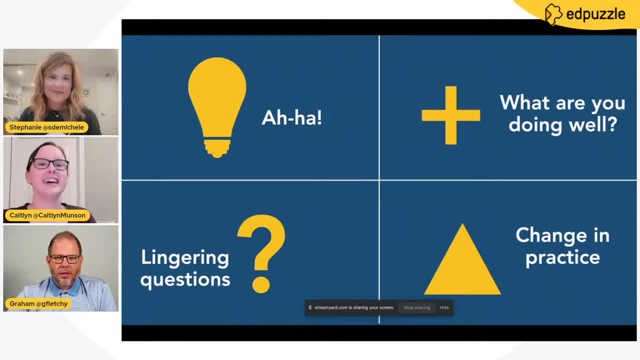 And I think asking: what do you notice, What do you wonder, Those questions can be some of the most welcoming questions. Yay, That's a reading thing too. That's a social studies thing too. I taught social studies once upon a time. 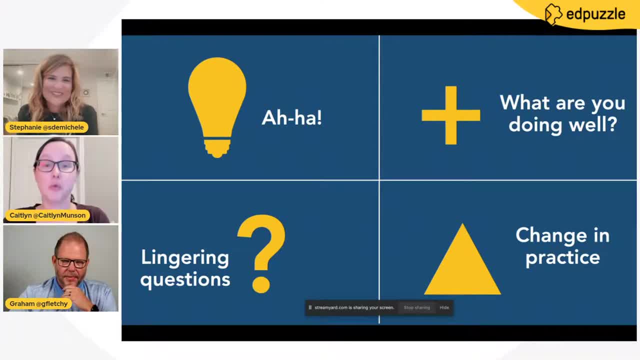 It's, yes, The crossover, the transferability. just the wonder: Yeah, absolutely, And I like that because it's not in a silo, It's like, well, this is the old. these are the questions I'll be asked in English. 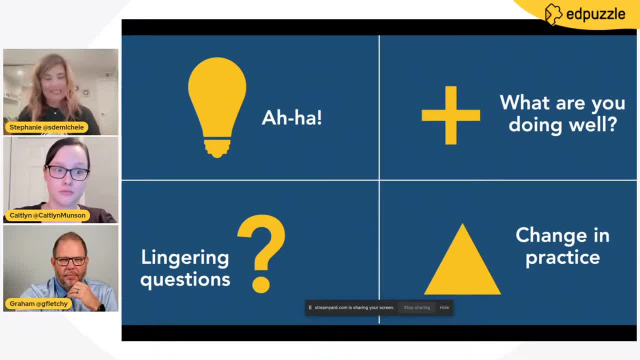 class, and then I'm going to go to math and have something different. It just all kind of blends together. Good practice for sure. Yeah, Manny, also made sure we. if you haven't checked out our Edpuzzle Originals yet, I certainly hope you will, because it's ready made videos. 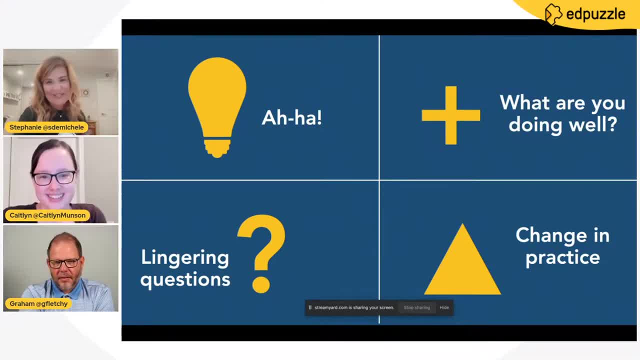 Grandma, here's another question I have since you mentioned at the beginning, because our students- this is this is the generation of kids we have- They love video, They love images. Do I almost see now kids going out into the world and seeing math now, wherever? 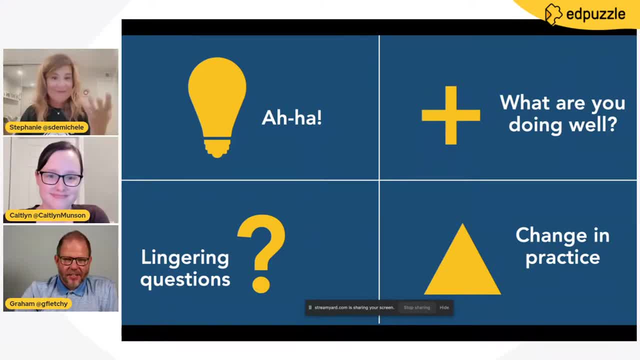 Now I'm never going to look at apples the same I am going to be looking at apples in a math minded way Do, I would imagine it's also probably a good idea to have students come with some kind of photo from the real world, an image and share out with the class, or 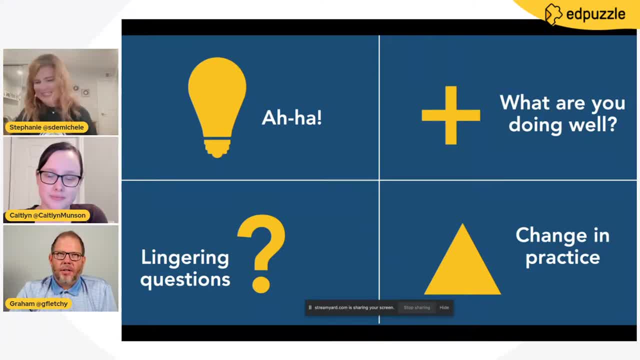 something like that: Yeah, So what you're doing there is you're giving students the power to realize that, hey, it's not just my teacher's class, it's ours, our class. So you can ask kids like, hey, well, you're, well, you're out this weekend. 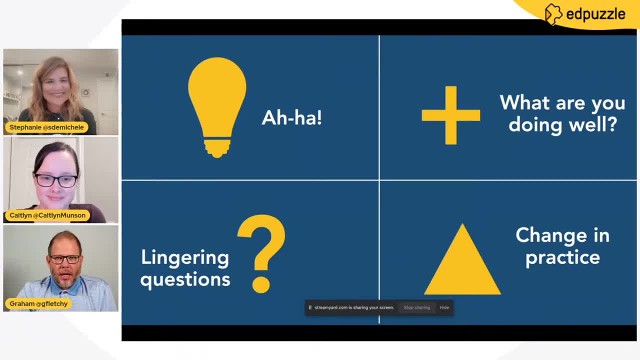 Your homework assignment is is when you see numbers in the real world. let your mom and dad take a picture. grandma and uncle, If you can capture a picture of it. I know our girls wouldn't have a cell phone in kindergarten, first grade class, but who knows what's going on? 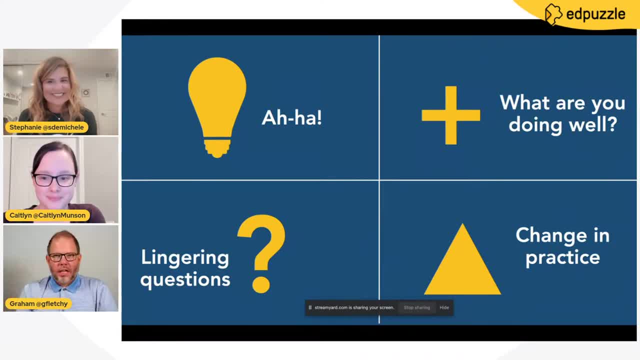 But yeah, get a parent to capture it and send it to you, Put it up on your projection screen and then let's not Student introduce the math that they saw and they can ask their classmates. So just seeing numbers in the real world. 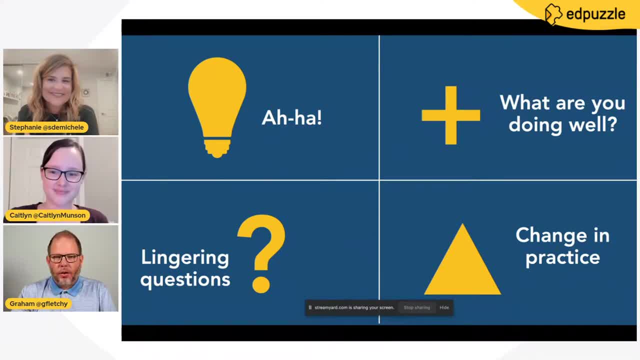 it's like mathematizing the world that's out there can be super powerful. Yeah, you agree. What you just described is our Edpuzzle student projects, which, as a math teacher and that math in the real world- I'm so excited about because students can. 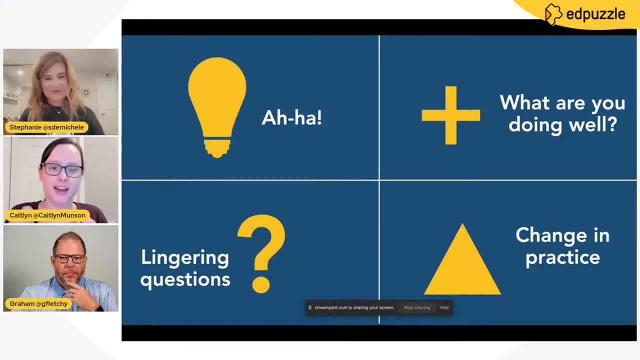 upload their own video so it can be something that they record with the class iPad or with their Chromebook or anything, And they can Go on, maybe a scavenger hunt around the room to find math in context, and then they upload that video and they can add questions and notes so they can. 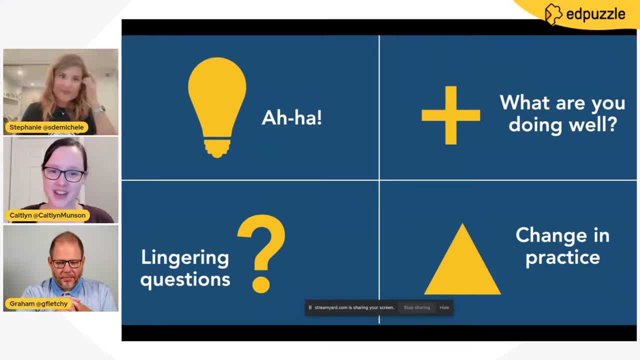 write their own math question and add it to that video And then you, as the teacher, can share that with your class and showcase that. Yeah, yeah, I am Joe And hi Joe. Yes, it's me. She said we did picture scavenger hunts last year for our notice and wonder which. 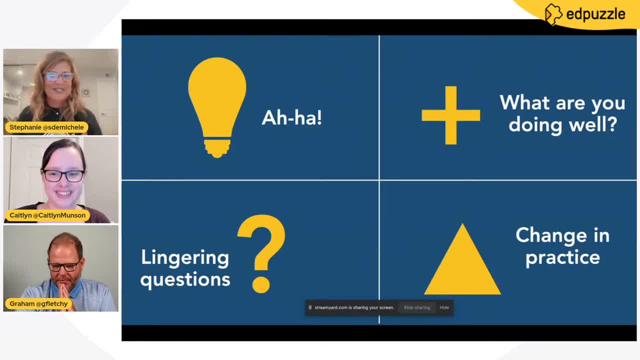 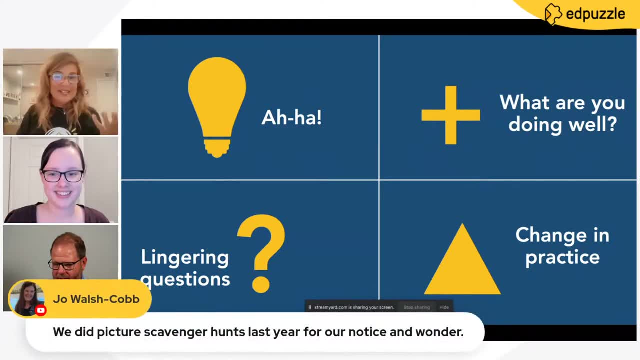 is genius, I think. Joe, are you still teaching fourth grade? You can drop that. there in the comments There's an Ohio girl, But yeah, it's that idea of the image, And so I guess the answer is the question when you say: well, when am I ever going to have to use this? 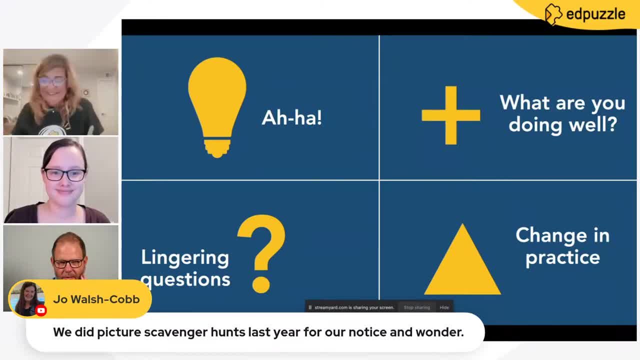 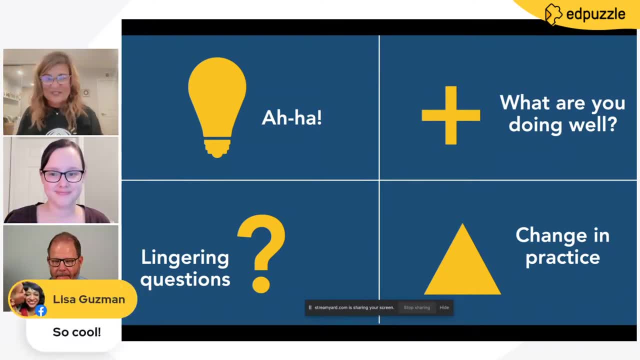 I mean, I almost think like, well, yeah, I don't know. I think it's amazing to be able to add the imagery to it. Yeah, Lisa, I agree It is pretty cool. So I think, whenever much is possible, 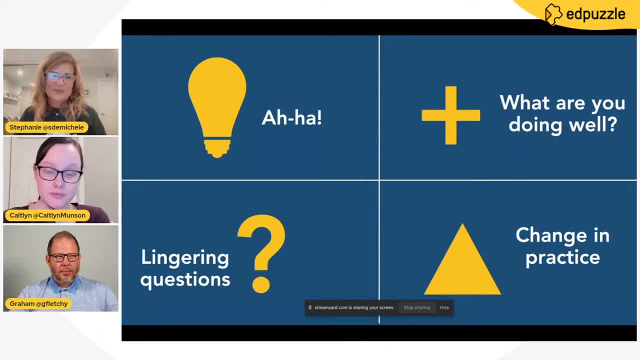 whenever, whenever I can, I always try and use media to bring what's happening in the real world into a math classroom, Like there's always going to be resources with lots of print for kids. Kids don't want print and print. It's really hard to make sense of print. 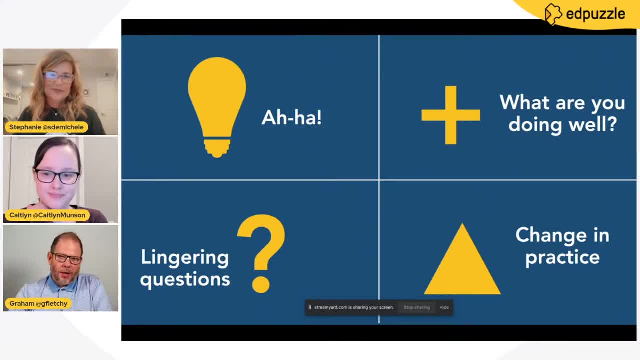 Now what will happen is, sometimes kids might have difficult with the print, but by introducing an image first and then following it up with the word problem, you're being really intentional and purposeful about making those connections for students, which is huge, which is a big piece missing for me. Yeah, 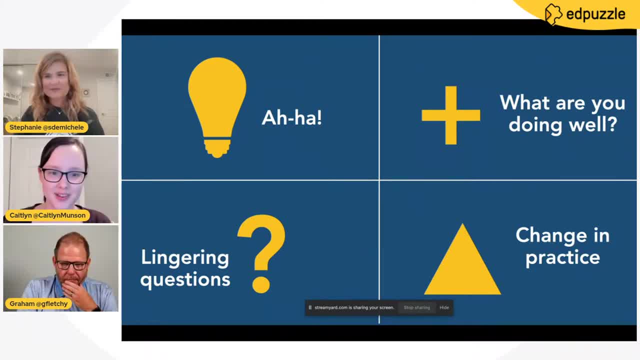 And it's also- I think Manny dropped the link in the YouTube chat. Maybe he'll drop it again- to the Edpuzzle originals which, when I saw your graphic where you were breaking apart your block, your where you're doing your multiplication, it reminded me of some of the graphics. 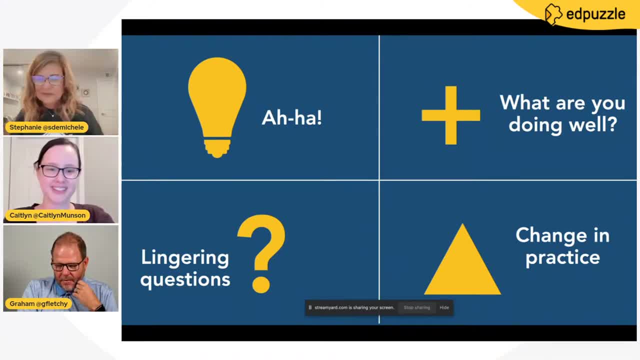 that our team has put in those Edpuzzle originals. There we go. There's the link If you want to check those out. they are currently available for all US teachers and then in our teachers joining us from around the world. 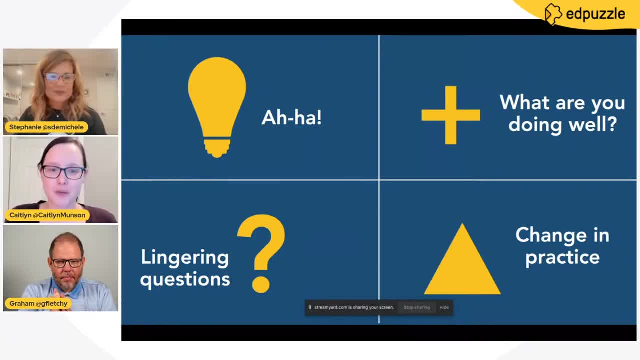 Right now they're available to pro schools. Check those out, Because it's really what you're describing And, in terms of connecting a word problem, which we know can be intimidating for our students of all ages and of all skill levels, and tying it into that graphic representation, but also multiple, 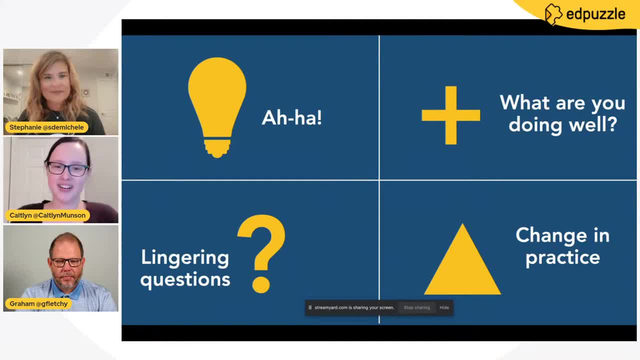 representations and and multiple algorithms, And oh, I just get so excited. Don't know if you can tell, That's how I look when I discuss Shakespeare, So I understand. So, all right, I think, Yeah, You had nice good vibes. 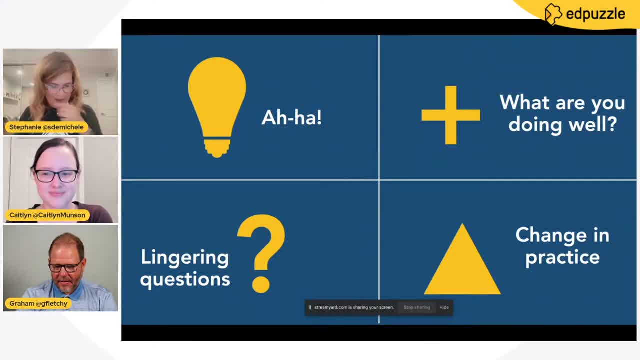 Thank you for everybody. I think I wrote this down as we were going through this. Here's what. here's my takeaway. I feel that math isn't something that's done to us. It's now something that we can participate in, And that was never. I always felt that math was something that was done to me. 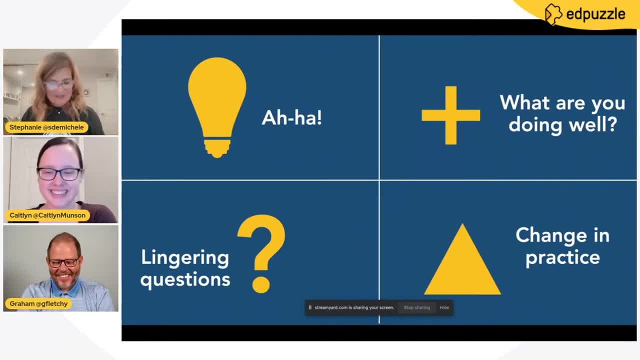 Awesome And I feel like an active participant, So I really I want to thank you. you, Graham, I want to thank all of you for joining us today, sharing these These amazing fact fluency ideas. Manny, if you could just one more time drop in Graham's contact info. 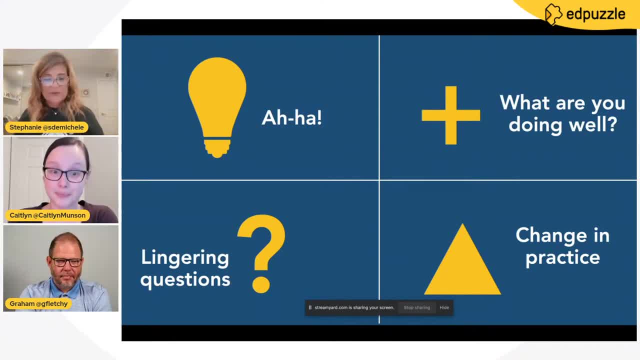 His website is chock full of the lesson strings. So, and as you go out into the world implementing these ideas, please share and post your own visual scavenger hunts, your fact fluency images, Please, please, please, share them out. Tag Edpuzzle. tag: Graham. 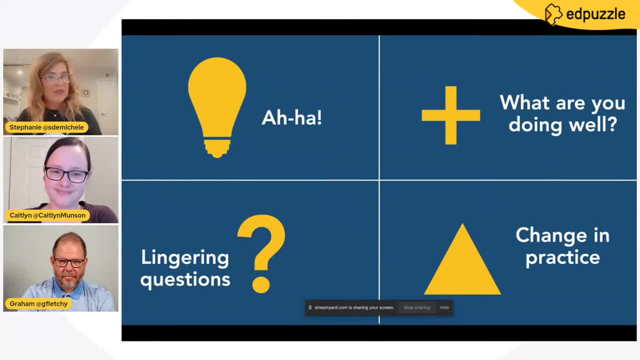 Use the hashtag: Edpuzzle live. We wish you a very happy Thursday. Anyone else want to say anything else? Graham, What else? you got Graham's having surgery by the most, So let's all wish him well. He's just torn Achilles tendon.